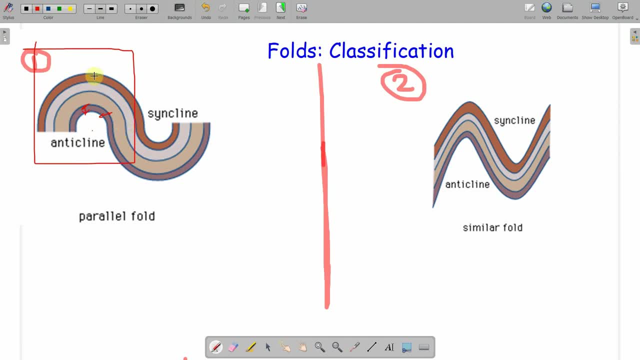 anticlinal bend is more sharper than the top portion. so if you move from this to this, okay, so at the top you'll be having a wider zone or wider area comparing to the deeper locations. okay, so, similarly for the synclinal, what will happen? it will become broader with the depth, but sharper. 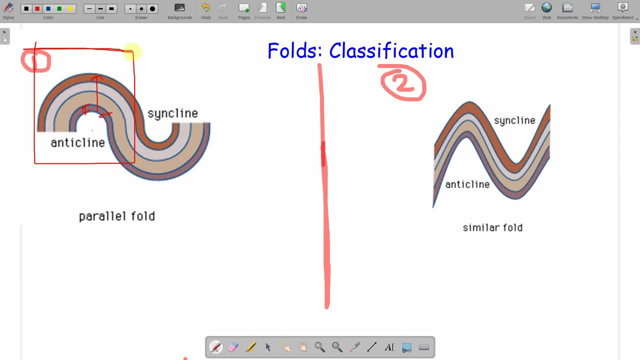 upwards. so what type of fold is this? this section, suppose you are seeing only this section, not not this one. so what type of fold is this? so what you can see it's anticline. okay, it's a symmetric fold. is it a symmetric fold or asymmetric fold? it's a symmetric fold, yes, and along with this: 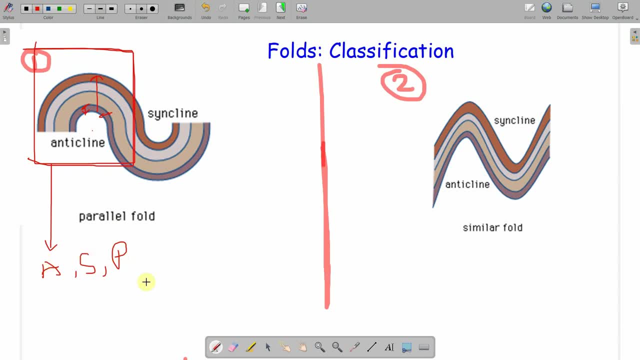 you'll be seeing, this is a parallel fold, so this is how you characterize any fold by stating these terms. i can understand so, okay. so this fold will look like this, so that in case of parallel fold, two things happen. that's, have a constant center, okay, and the thickness will be constant throughout the area. thickness of any layer will be constant. 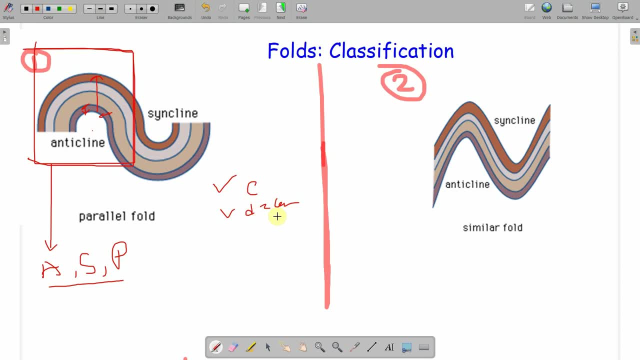 another type of fold or classification you can consider. that is the similar fold. so in this case the shape of the folds may vary. in this case the shape will be varying. whatever the shape will be, the shape will be varying. okay, and and at right angle, very among the axial plane, and also at the right angle of the axial plane. 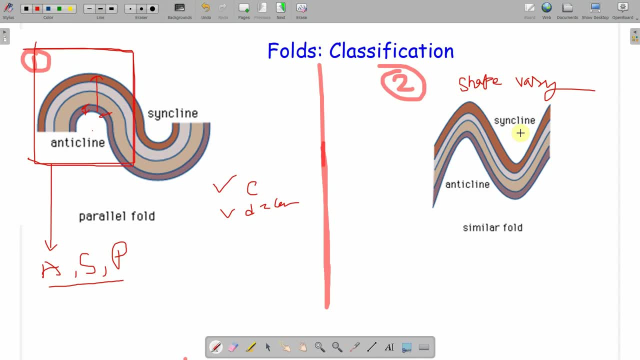 both sides the shape will be varying. and here every bed is thinner in the sampling portion, so here you can see the border Jahrw. at the limb portion the bed is thinner and thicker at the hinge portion. so, and in the hinge area the bed will be thicker near the hinge and bed will be thinner throughout the limbs. okay, so for this. 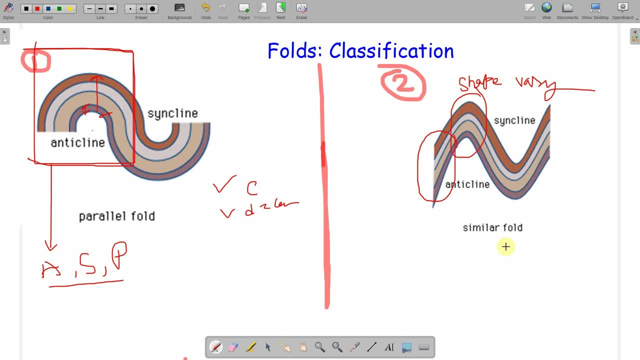 there must be a considerable plastic movement of material away from the limbs, which is so plastic. what happened here? the plastic material will be moving from this portion and it will be depositing this point. so considering the thickness of the limb, thickness of the limb we can classify parallel. 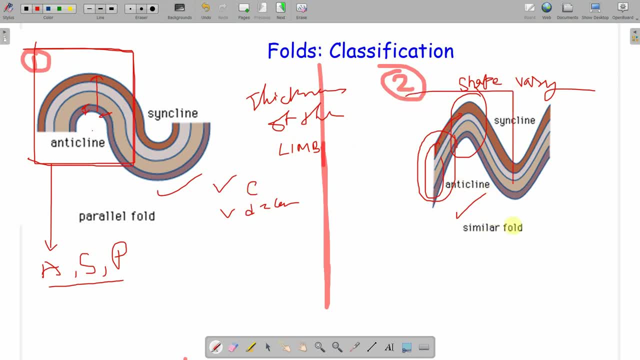 fold and similar fold. so what type of fold is this? if i take this core section or if i take this section, so this fold is your anticlinal first, and this will be, uh, symmetric and it's a similar fold. okay, this is how i will be mentioning any fold. now, another type of case you may observe: uh, 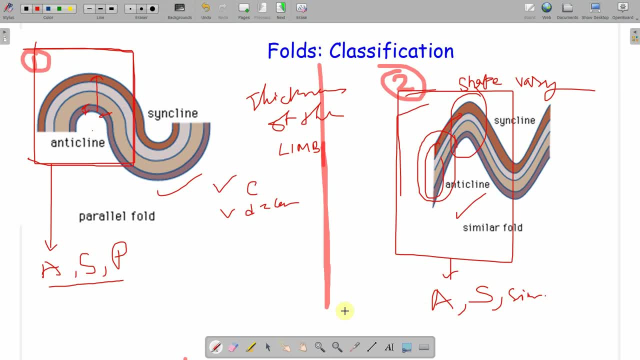 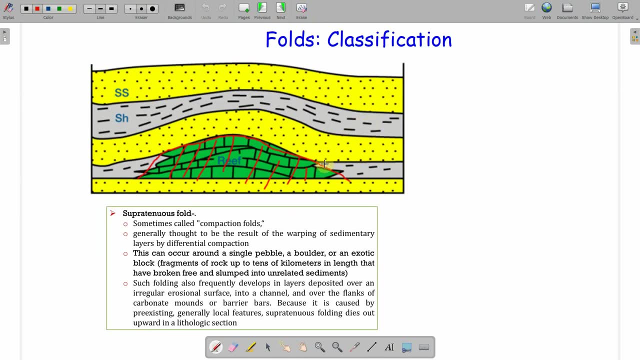 and you may classify a fold with the basis of thickness of the limb. there is another type. there is a third type that is called the suprataneous fold. so in case of suprataneous fold, what happened is sometimes called the complex in folds. so see this rift reef structure, remember so it's. 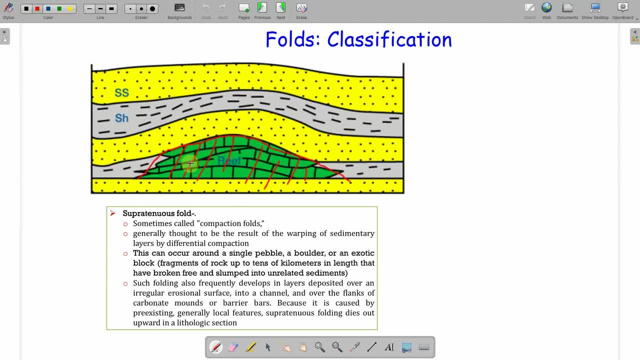 a mound like structure. it's a pre-existing structure of Dinge gave constitution of the territorial structurelegtric structure of a flexibleYes, sorry, with nearly dispersed so that it cannot fold. a structure generally is thought to be the result of wrap, wrapping of sediment layers by different 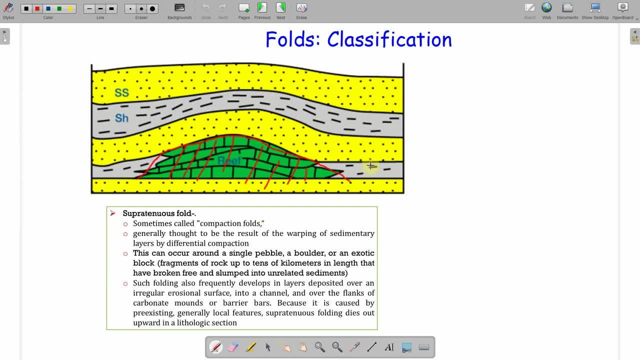 differential complexion. i'm coming to that. so how this is formed. first let me explain the suprataneous fold. suppose there is a mound like structure on a on earth surface. this is the mound like structure, or this is called reef. now sediment depositions are happening. so how the sediment deposit, sediment will be deposited. 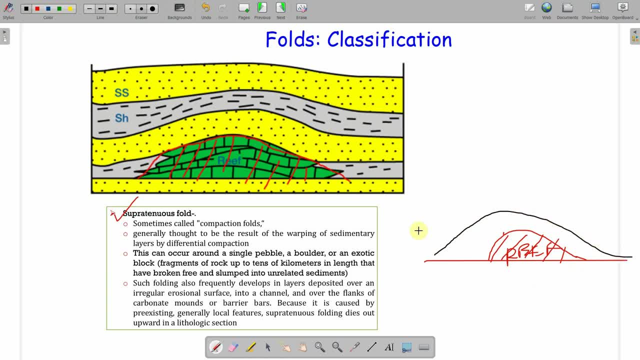 like this way. like this way, then another layer will be there. so, in due to the presence of this structure, you are having the folded structure. i'm not drawing it properly, okay, so like this. so suppose, uh, one year, the river walk or anything for any physical agency depositing sediments of this is the, let's say, this is sand and this is. 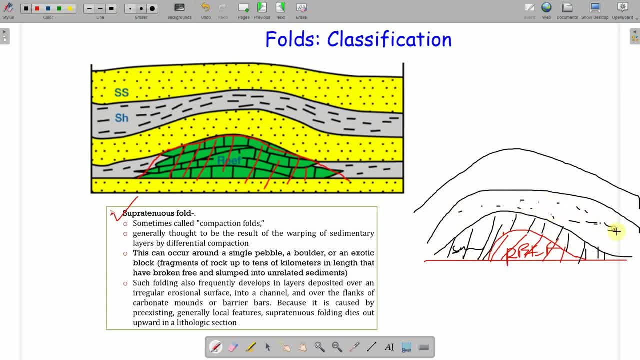 shell has been deposited later. this is shell. then again sand has been deposited- sand layer- and after compaction you will be seeing a folded structure. and that fold is only because you have a folded structure. and that fold is only because you have a folded structure of the presence of this reef structure. so this can occur around a single pebble bolder or 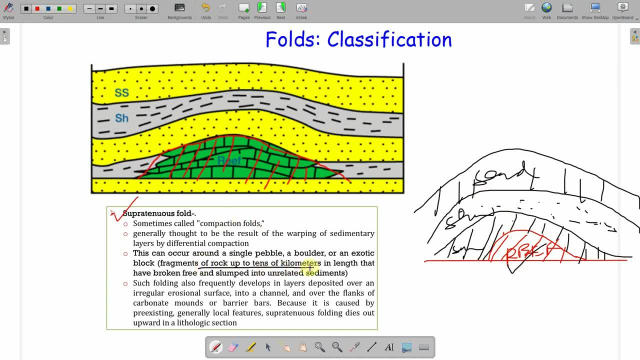 an exotic block of the fragments, and when i'm talking about the boulder or any exotic block or any existing rock, rock body, that rock could be of tens of kilometers, it could be 10 kilometers in length, so the structure it will create it to be above it will be huge, okay. so such folding also. 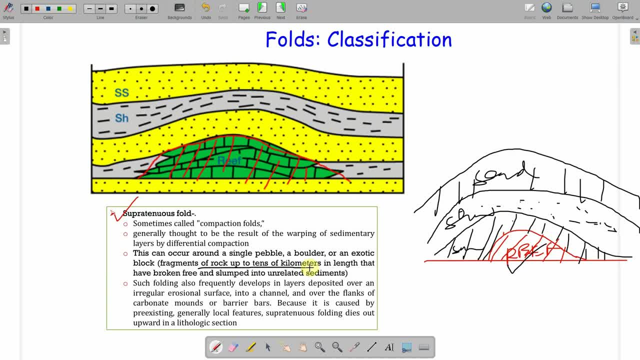 frequently develops in layer deposited or irregularaban seu naft一点 geoforum layer depositate order, irregular erosional surfaces. and one more thing i didn't describe here that: the differential complexion. what do you mean by the differential complexion? so after sedimentation, that means the accumulation. 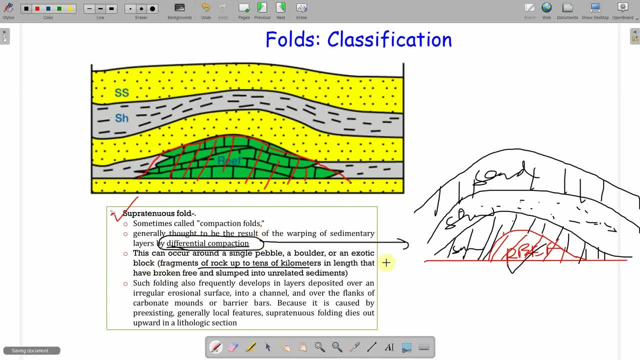 of sediments after sedimentation. what happened? the complexion happened and other chemical precipitation, uh, cementation. these things have happened. but the main part is there is the complexion by complexion or uh by complexion, um, uh, a sedimentary rock form, and how this complexion or this pressure you are getting. this pressure you are getting from the overlying load. 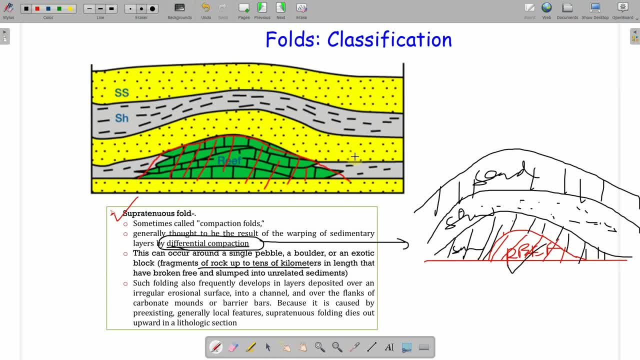 so by differential complexion means not everywhere same type of complexion is happening. for this reason, what may happen is that the strata is thinnest at the crest, like this, this layer, consistency at this level, others- i cannot draw it properly. so consider this layer. from here you can get an idea that at the case it will be the thinnest. 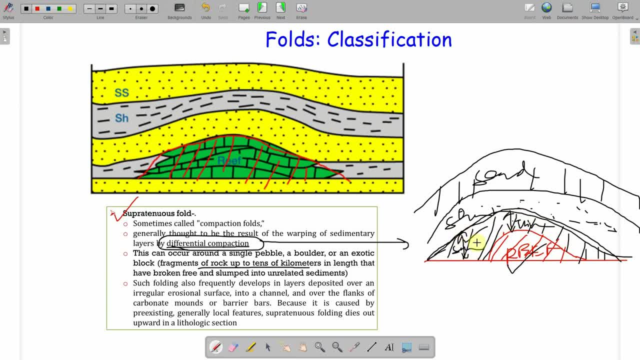 and at the, at rest of the portion or at the limbs portion, it will be the thickest. okay, so for the anticlinal structure, it could be anticlinal or it could be like it's in planar. so here are the strata at the thinnest, at the crest of the anticlines. okay, so this will be. 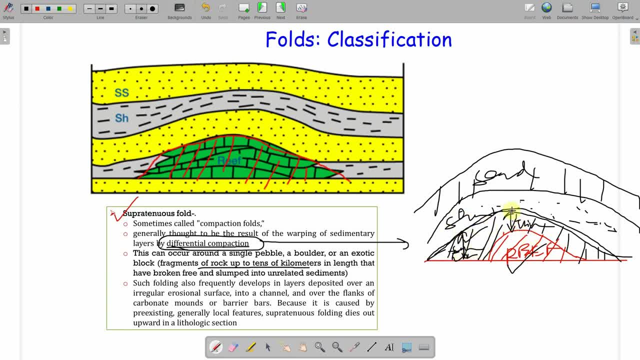 the thinnest and the thickness here will be better than this portion, okay. the opposite thing happened for the synclinal condition also. if there is a basinal uh structure, okay, if there is a basin like section, then there will be deposited and the folder structure will be developed, so that that is also quite common. but 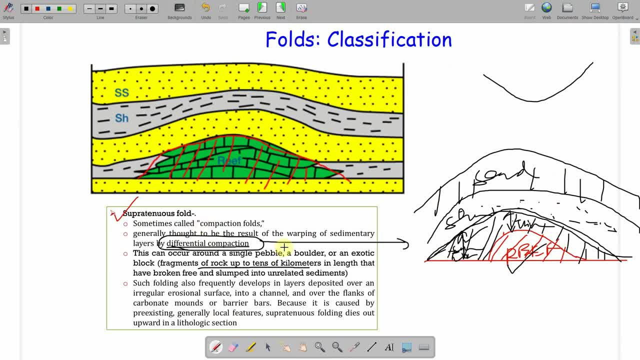 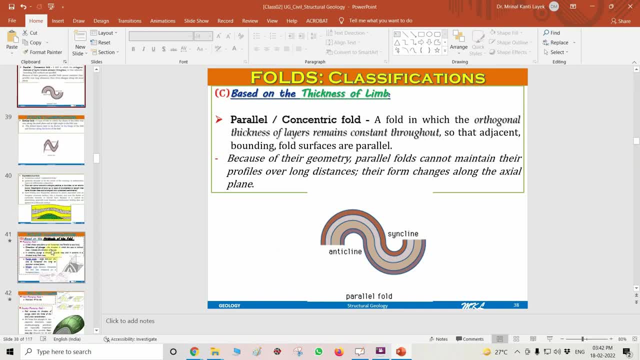 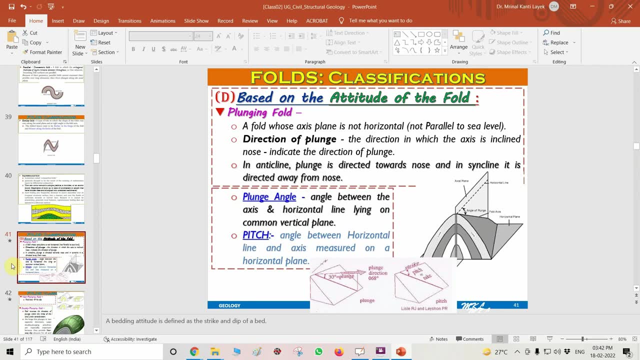 this type of structure is generally called the supradaneous fold. okay now, on the basis of, on the basis of attitude of the fold will be classifying fold will be classifying the folds on the basis of the attitude. so what do you mean by attitude of the fold? attitude means strike and dip of a plane, if I 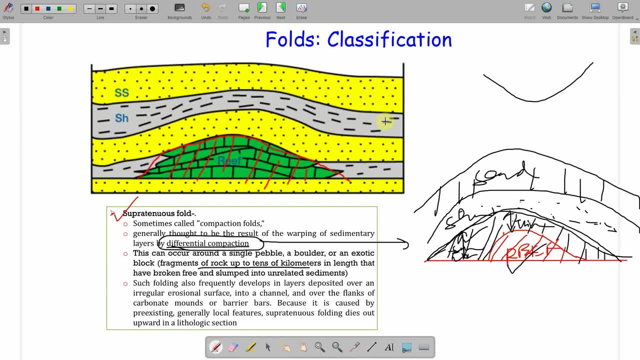 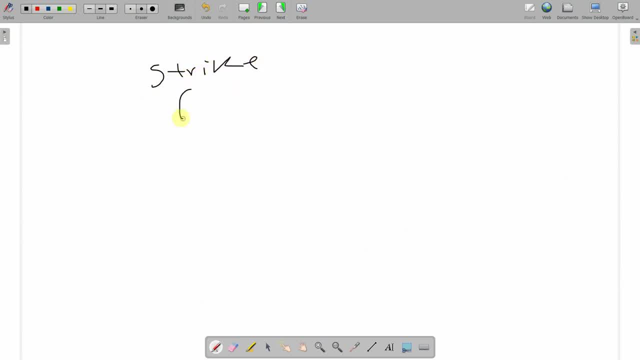 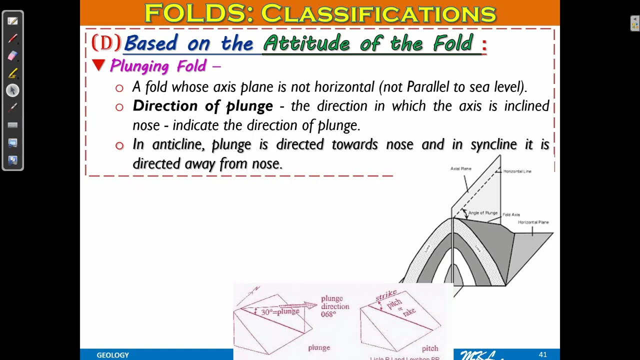 talk you about the attitude. attitude mean is called the strike and dip of a strike and dip of a bed, of a bed, is called attitude. okay now. so, depending on the attitude of the, depending on the attitude of the fold, you can also classify folds into several types. typically, five types folds have been recognized on this basis, 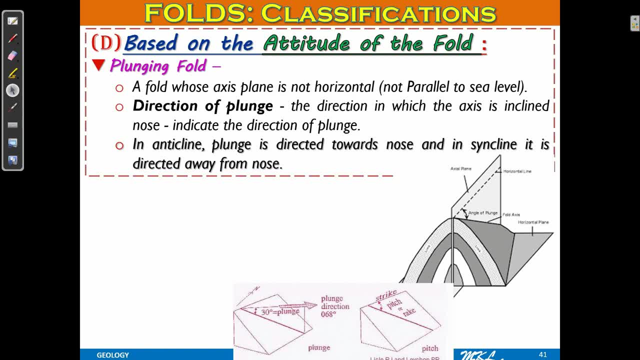 first one is the plunging fold. a plunging fold is that fold which has a axial plane or the fold axis inclined with respect to the horizontal line, if the fold axis is plunging. so what do you mean by plunge? plunge means that the angle of inclination- Apple now suppose this is the horizontal line, and 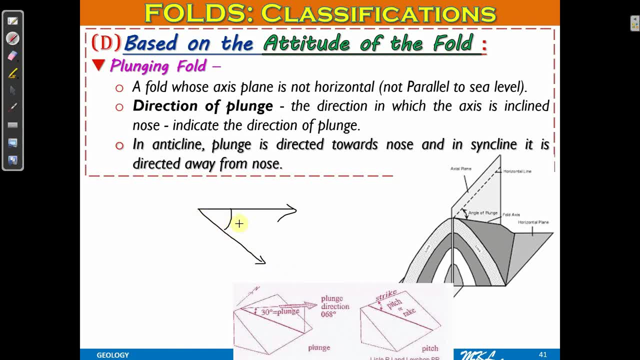 there is some inclination, any linear features or anything. okay, so if this thing happen, this angle is called the plunging angle. okay, so this angle will give you the sense of plunging and this inclination is called the plunging. so if your fold axis, if inclined and making an angle with the horizontal line or the 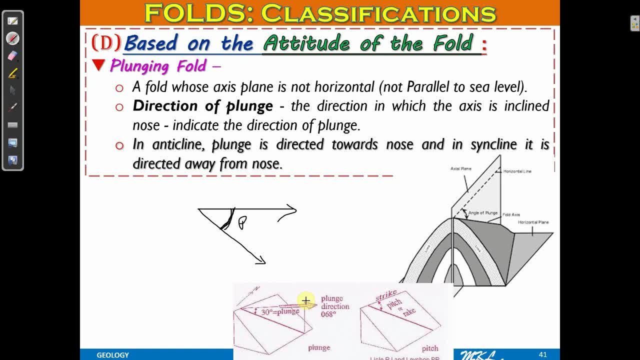 horizontal plane, then you will be seeing or saying that that fold is a plunging fold. okay, so in a anticline, plunging is directed towards nose and syncline is directed away from the nose. so these structure, this folded structure, is exactly look like nose and by seeing. later I will discuss how you recognize a 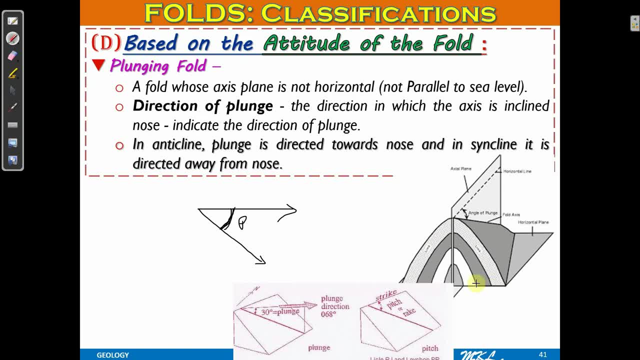 fold in field, there will see that this nose is kind of structure, is very prominent to understand the folded, to understand the fold or the fold. structural mapping so in anticline plans is directed towards nose and syncline it is directed away from the nose. okay, so if there is a inclination, if there is, 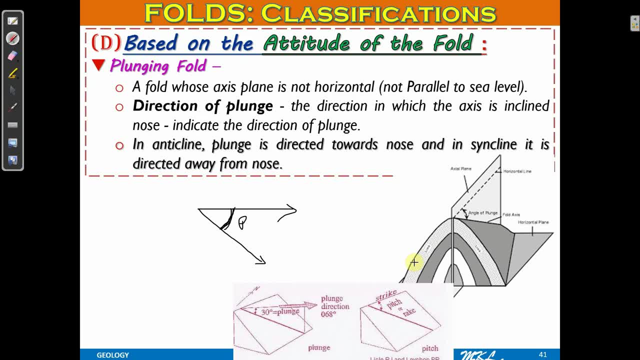 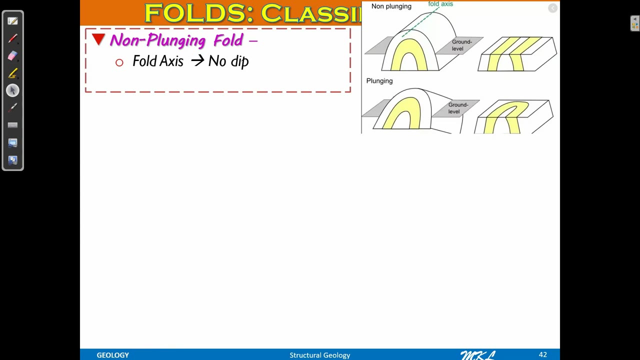 inclination from the horizontal line, that's called the plan. if fold axis is plunging is called the plunging fold. same explanation for the non plunging fold. whatever the fold, the regular fold I was drawing from the day one that fall was non plunging fold. what do you mean by non plunging? 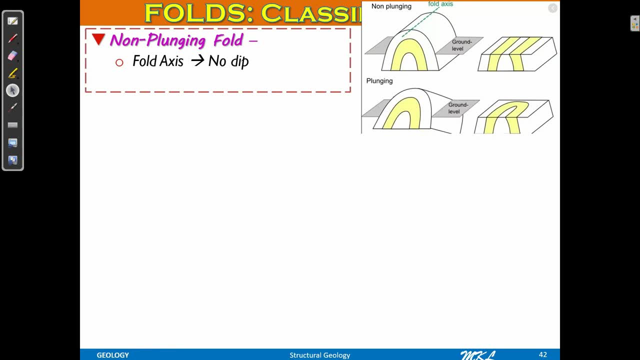 fold when the fold axis is not plunging. so here you can see the fold axis is plunging and it's making an angle with the horizontal line. but here you can see the fold axis is origin. sorry, a full plane is the horizontal. okay, so the fold axis. okay, so the fold axis is horizontal. if you draw a axial plane, you 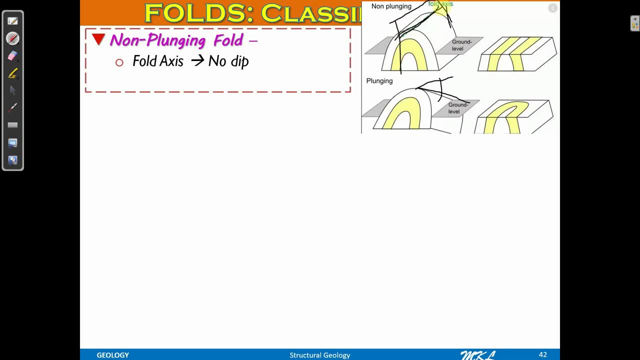 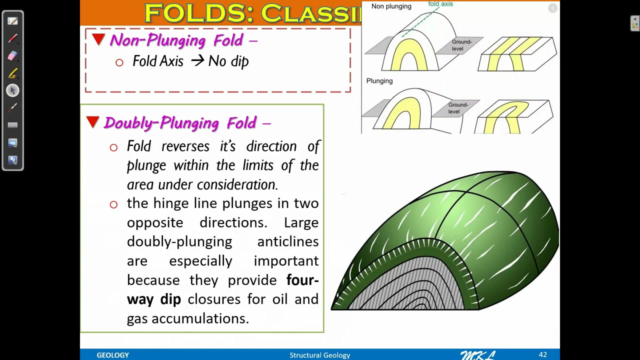 will get a axial plane like this. so here the fold axis is horizontal and as it's not plunging, that's why it's called the non plunging fold. and as it's fun, plunging is called the plunging fold. as simple as it is. now there is another type of plunging fold you can identify. that's called the. 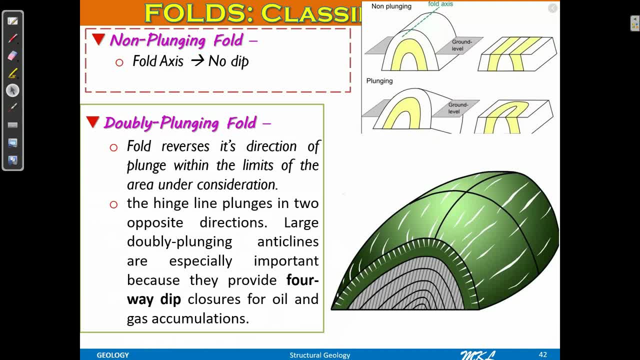 doubly plunging, fold it kind of. it may be looking like a hole, malum and a hole okay. so if you cut the hole in a half it will look like that: dole malum a kiss up this ago. dole malum a dole, malum a kiss up this ago. dole malum a kiss up this ago. dole malum a kiss up this. 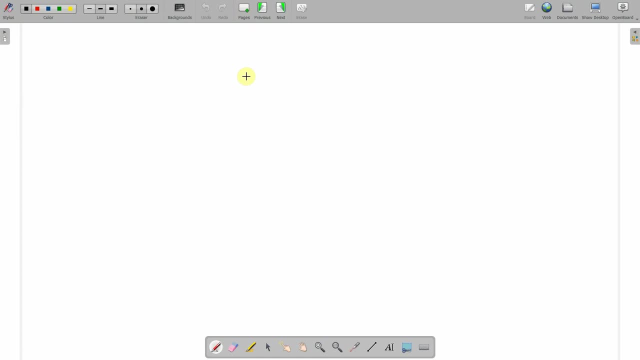 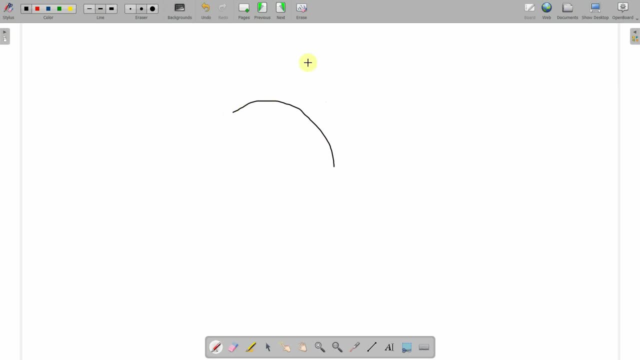 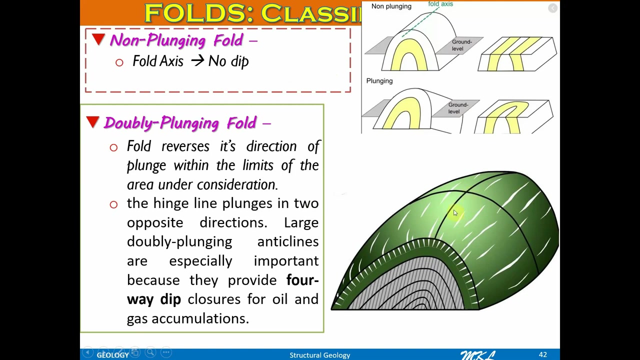 plunging direction. you can see one in this direction, another one in this direction like this one. see, see here, if I've taken, I take this is an axial plane. okay, so this fold axis is dipping this direction, in the front direction. this fold axis is dipping that direction. so there is a plunging. it's deviating from the horizontal line or horizontal. 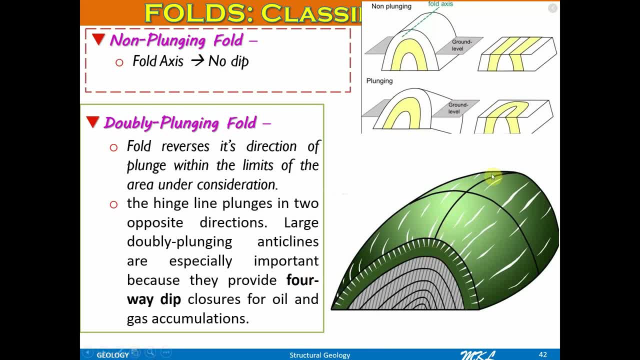 plane but it's plunging in different direction than the others. so fold reverses its direction of plunges within the limits of the area under consideration. that's like a top surface of a fold. that's kind of example of the w plunging fold and the hinge line plunges in two opposite 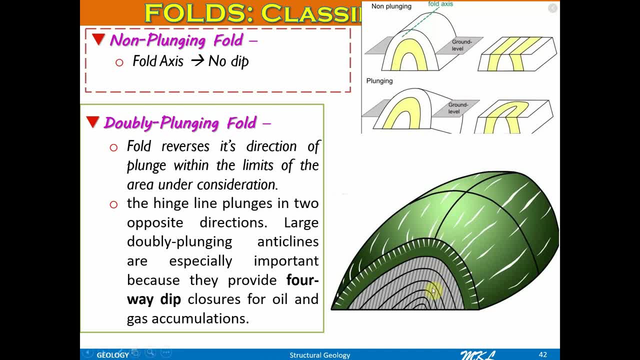 direction, for obvious reason, it's plunging in the front direction, it's plunging in the back direction, so this line is dipping in lemmings term, or in simple term, this line is dipping in the front direction, this line is dipping in the opposite direction, as there is double plunges, are there? 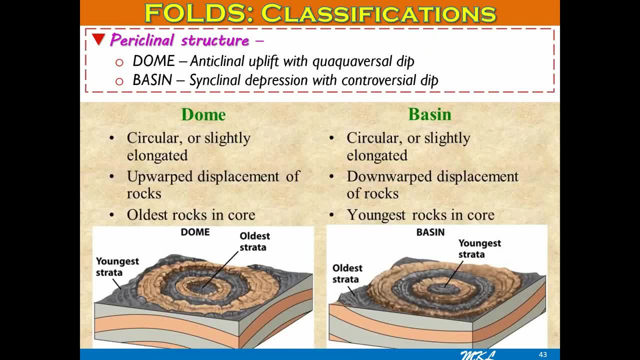 that's why it's called the w plunging fold. so now another type of structure you will be seeing, or another type of fold you can see under this classification, under the classification attitude of the fold. so we are discussing about the attitude of the fold, the abstract and deep conditions of the fold. so, depending on the 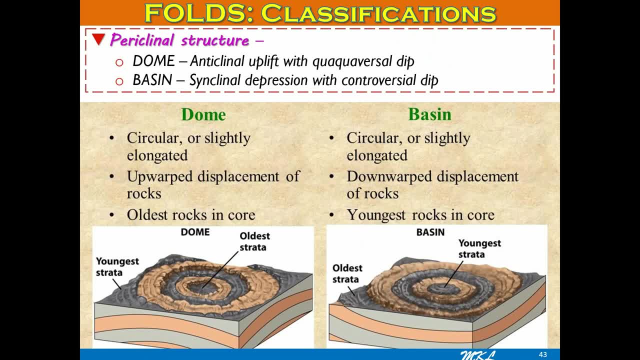 attitude, I am classifying these things. and fourth type is your periclinal structure. so periclinal structure basically can be classified or can be recognized into two types. one is dome, one is basin. dome means it's a mound like structure. so when it's a mound like structure, what 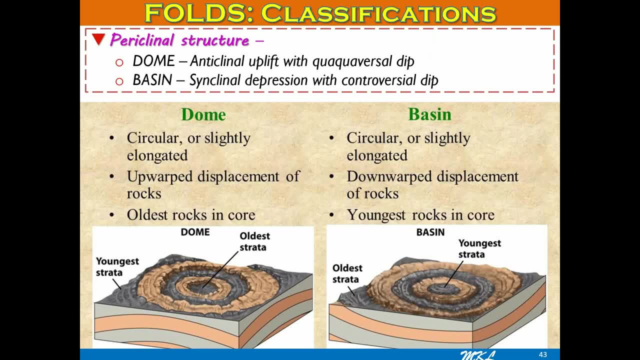 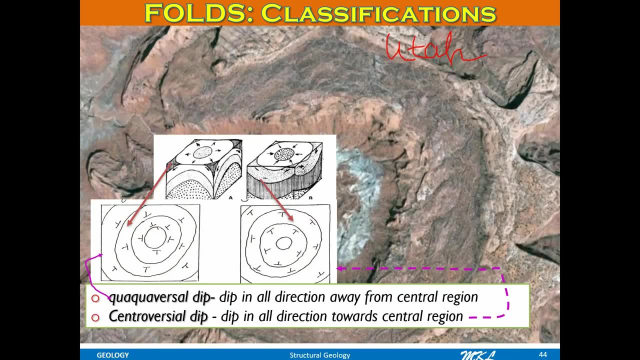 will happen from that portion, from the centre, the structure. if you do the structural mapping like this, if you do the structural mapping and it's a mound like structure or hill structure, then what will happen? this deeping will be from the centre- is called the periclinal grip. for further, for the 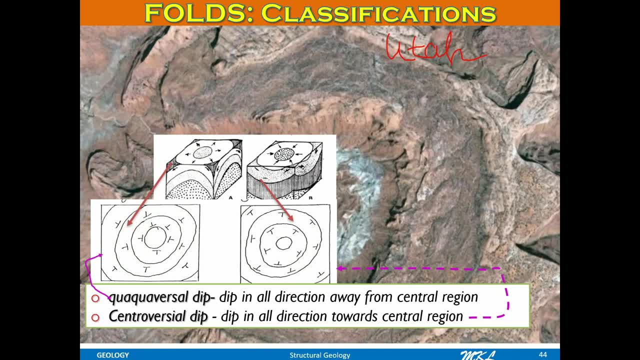 so this triplat quality, which is the quality of scopizing, that should be kept. I did not put out but what I did, just save this. but if you would focus on the structure, then what you will get is the never be shaped. if you so, both the neck and blade can be medicate�. these are kind, first step, and I change the focal device before you get them, while switching between bottom three and left, after a dive heart by example, personnel deposition ofshaped door. so for this, if you would increase, divideShow house. 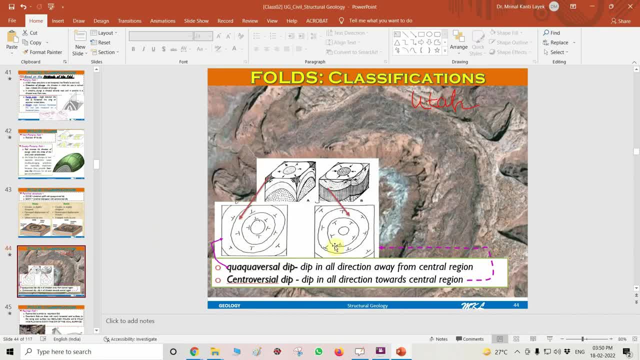 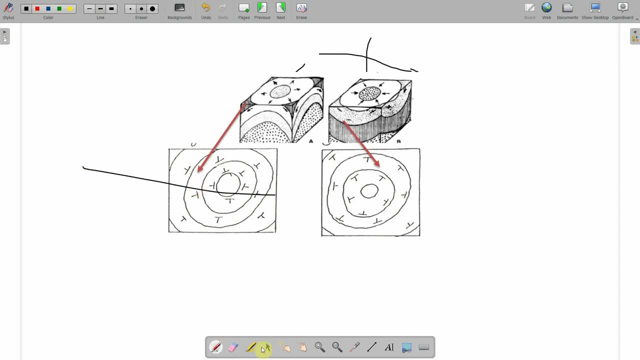 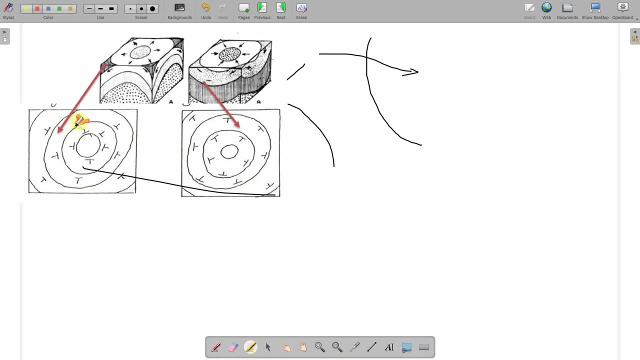 let me first explain. let me explain this. what do i mean by this? okay, so what does this mean? this t? okay, so this t means this is the strike direction and this is the dip direction. you know that the strike is dip is perpendicular to the strike direction. 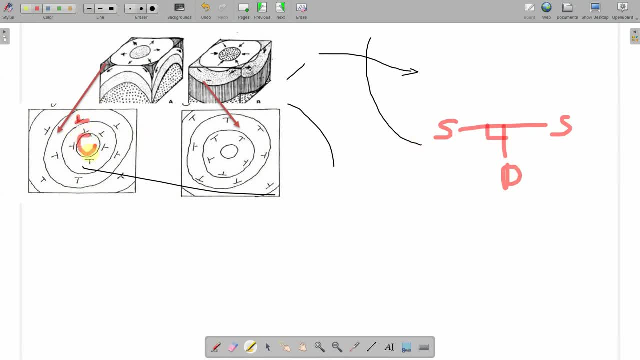 okay. so here you can see from the center position the deep the dipping case is. uh, or the strata or the bed is dipping away from the center position. okay, just like a bound like structure, that's called the dome. if this is a crater-like structure, that's called the what is called basin? okay, so 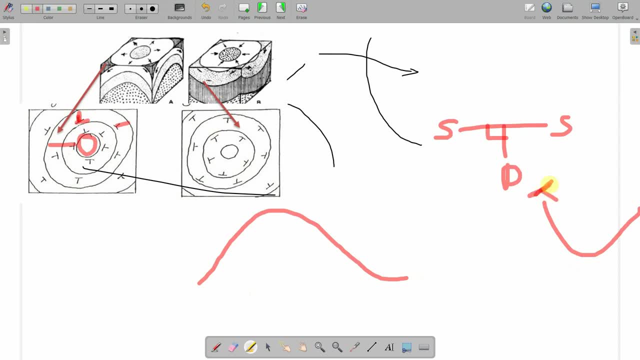 in the basin test. you can easily understand that if this is the strike direction, this is the dipping. dipping will be to the center, and here the dipping is away from the center right. so this dip is called the coir-coir versile dip. this dip is called the centro versile dip. 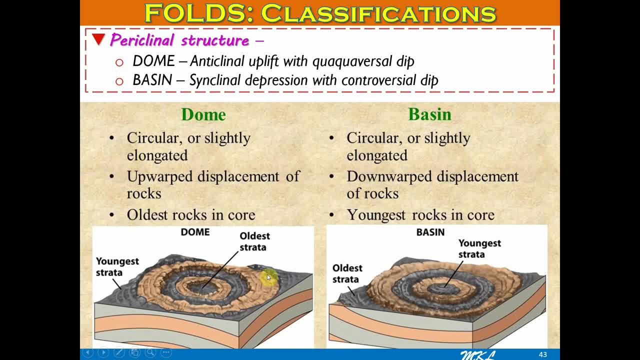 and you will find old strata in the core. for the dome condition for the basin case, you will find young strata in the core. okay, so here, up wrapped, displacement of the rock you can see. uh, in the basin case, down wraps, displacement of the rocks you can see. so dome 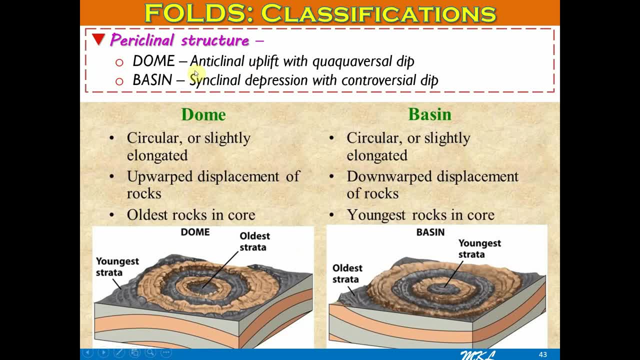 is kind of a anticlinal uplift. suppose a uh, a small mound is going up and it make a folded structure in the surroundings that's called the dome, and if there is a like crater, volcanic crater is there. so if that structures, you might have heard of eye of the earth in the sahara desert. 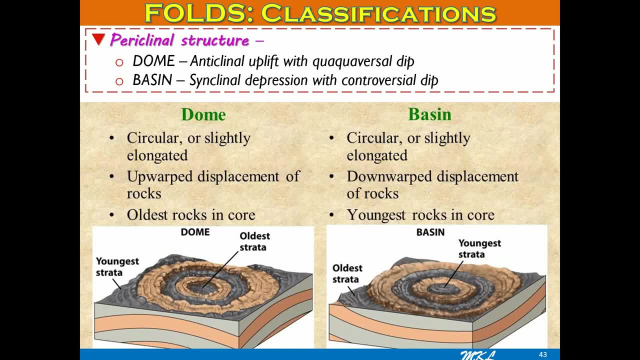 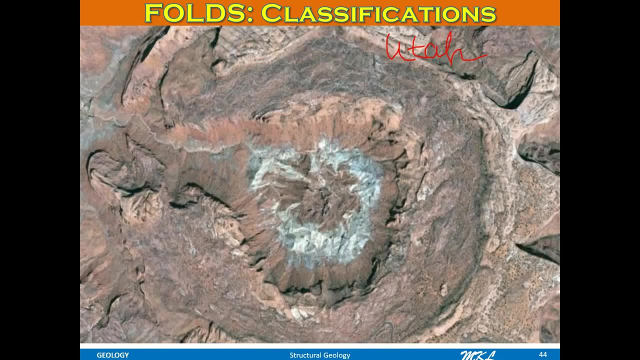 that's basically the dome structure. eye of the earth. have you heard anyone? eye of sahara, not eye of the earth. eye of sahara it's called. it's actually a dome structure which is quite visible from the satellites. okay, so this is an example of dome from utah. 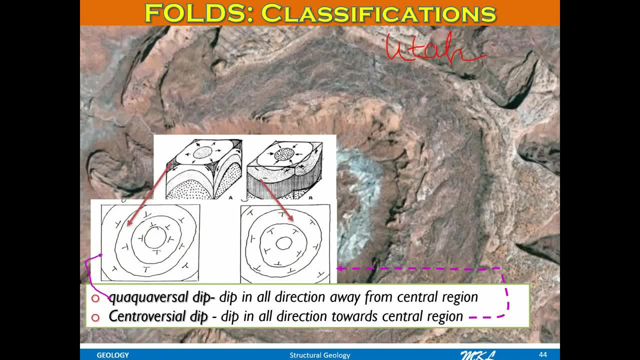 and so what is the coir-coir versile dip? this type of dip is a coir-coir versile dip, okay, so where the dip in all direction away from the central region is called the coir-coir versile dip- centro versile dip- is the dip in the all direction towards the central region is called the. 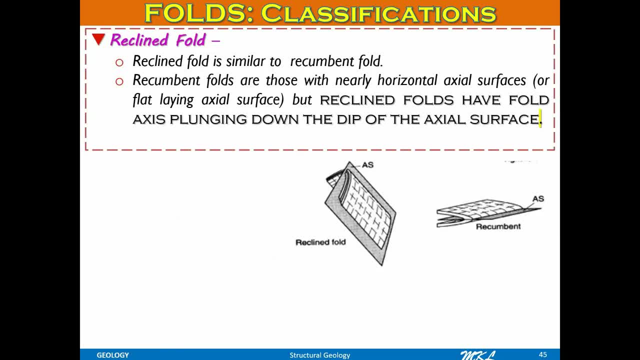 centro versile dip. now, most important part of this classification is the recline fold. so recline fold are almost similar to the recumbent fold. but what is a recumbent fold? if you recall, the recumbent folds are those which has a nearly horizontal axial surfaces like this: if the axial surface 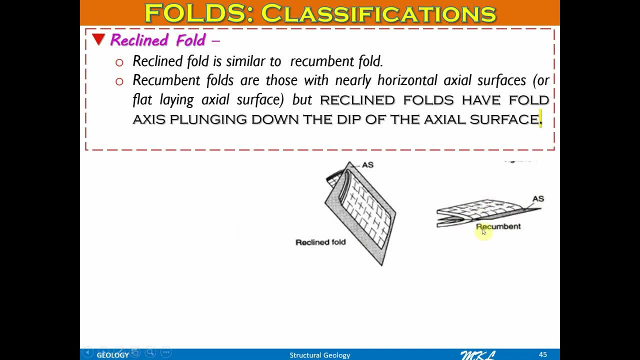 is horizontal, then it will be called as a recumbent fold. but in case of reclined fold, remember this very carefully because i'll ask you about this later- i'll be presenting some, i'll be presenting some photographs and i'll ask you, so be ready with that. these suppose this is the 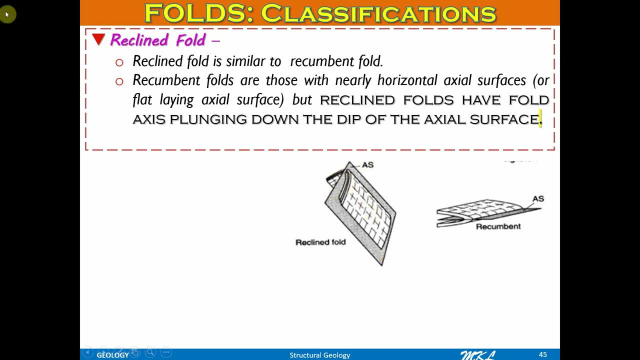 axial plane of this fold and as you can see here that the axial plane is dipping this direction and in the same direction the axis is also dipping. so the recline force of fold axis plunging down the dip of the axial surface. if i refine this thing, that hinge line you can see the hinge line is dipping along the axial plane. 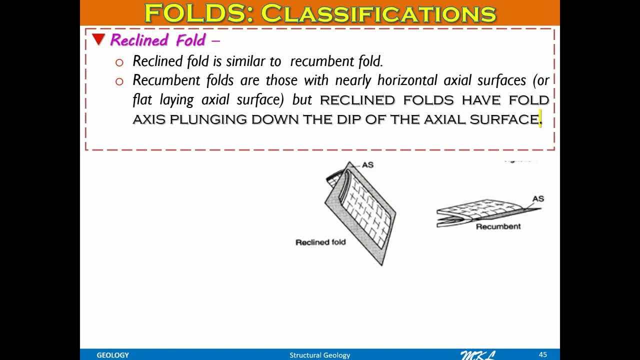 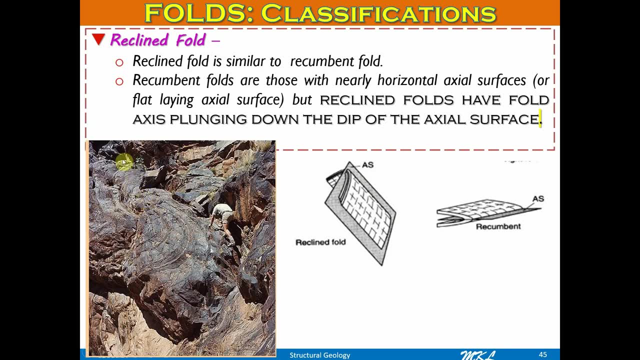 that's called. that type of fold is called the recline fold, so this is an example of the recline fold. the entire axial plane is dipping this direction and the axis is also dipping in the same direction. not dipping plunging. plunging should be the accurate word. 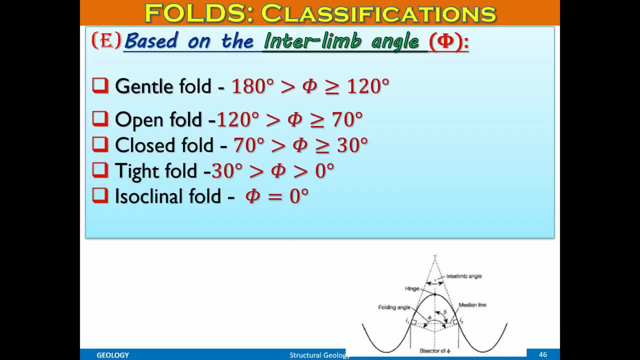 now based on the interlimb angle. so what is the interlimb angle, anyone? what do you mean by interlimb angle? what do you mean by interlimb angle made by the tangents? from which point i will be making the tangents from, from the infection inflection point, from the 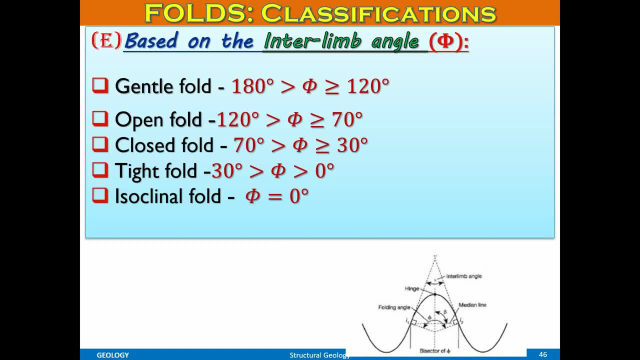 inflection point. you remember the inflection point, right where the sense of curvature changes. okay, that's the minimum curve point, or minimum minimum, that's the point where the curvature is minimum. that's the inflection point and from that point you will be drawing some two drawing. 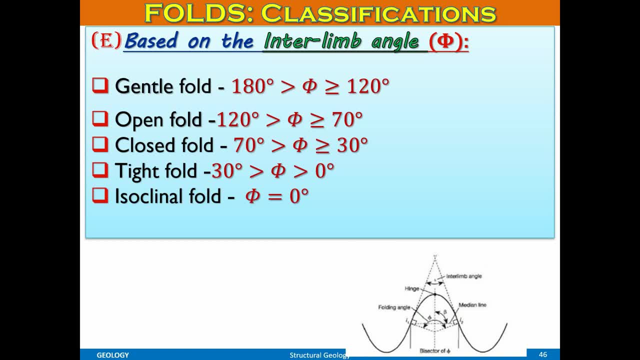 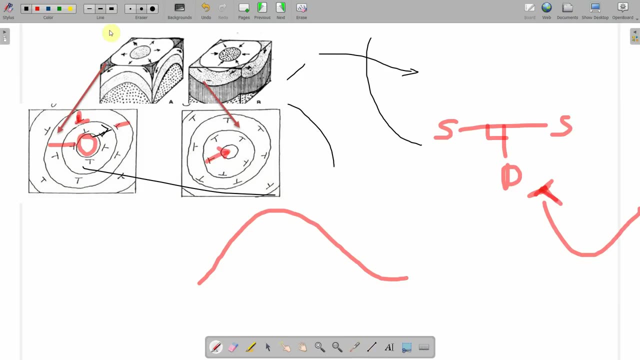 tangents and that will be intersecting some point. so gentle fold is 180 degree to 120 degree. okay, that's a kind of wide light structure like this. so this type of fold would be your gentle fold if i draw this structure. so if i draw, 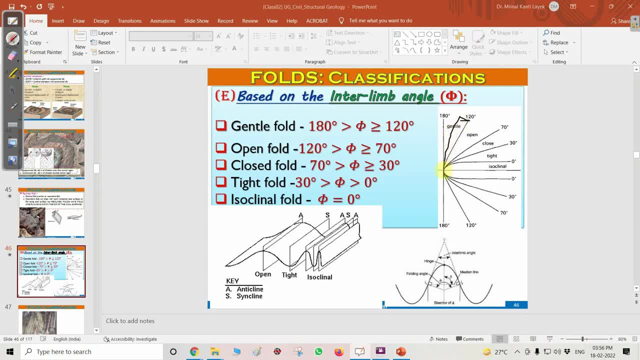 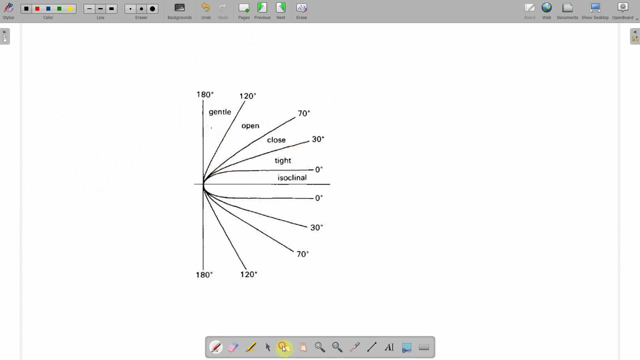 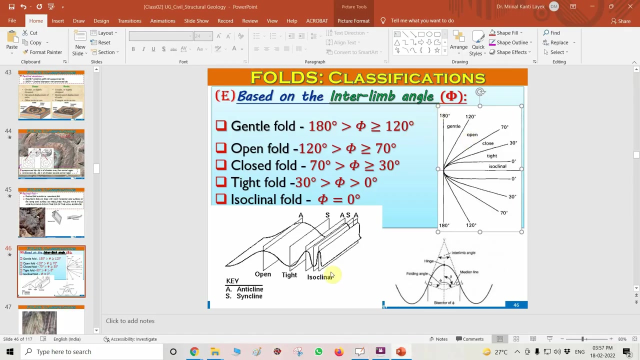 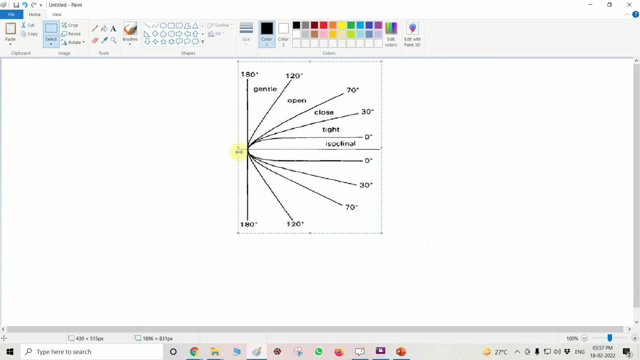 the folded structure here. yes, of course you are not understanding. let me take it outside, okay. um, how i can rotate it? okay, Give me a minute. Yes, So I have rotated it. So what do you mean by gentle type of fold? So I am considering that the 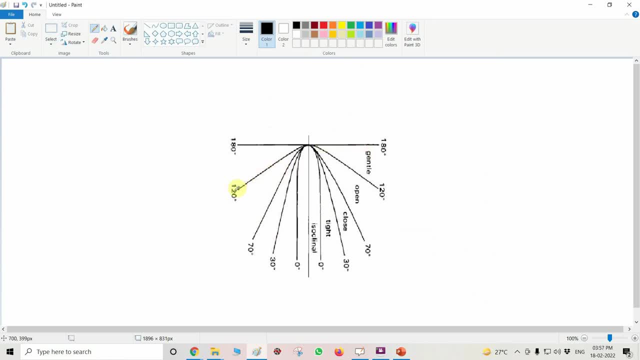 interleave angle is 120 degree. So if you draw it, okay, One folded structure, You got the idea right For the isoclinal, how I can draw it. So that could be the isoclinal, That's the isoclinal. So if I take this, 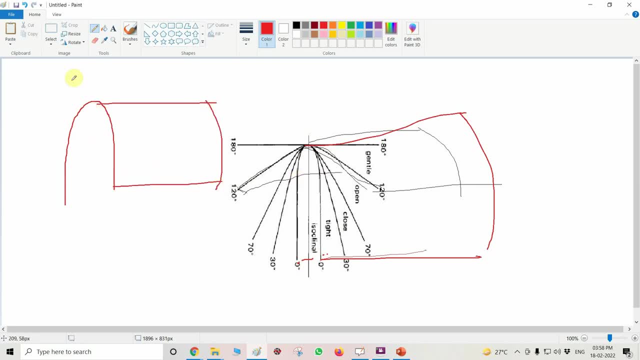 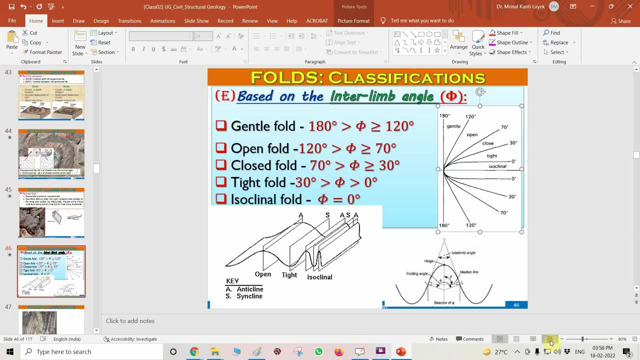 this is kind of isoclinal. So isoclinal means when this angle is 0 degree or near to 0 degree, That's called isoclinal. So depending on the interleave angle phi, we are classifying the fold into 5 types: Gentle fold, where the 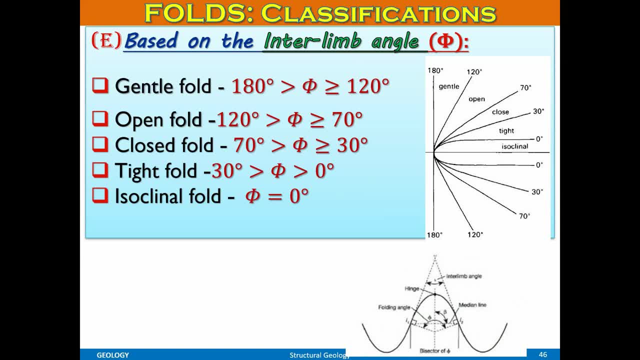 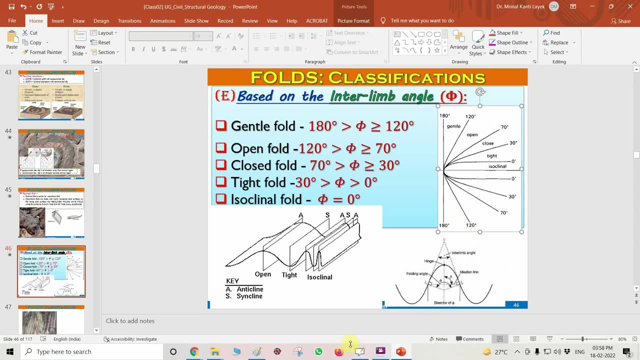 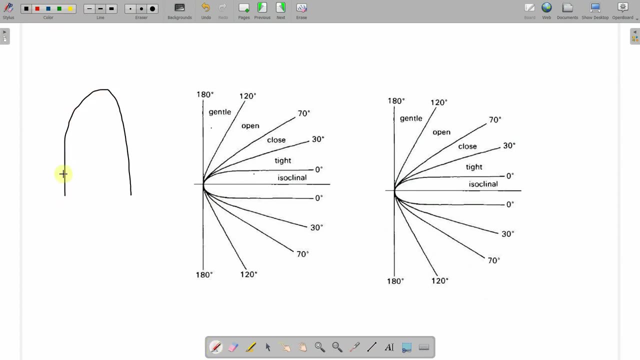 angles are in between 120 to 180.. Tight fold: 0 to 30 degree and isoclinal fold when the when both the limbs are parallel. When both the limbs are parallel, then I am saying when both the limbs are parallel to each other, like this. So 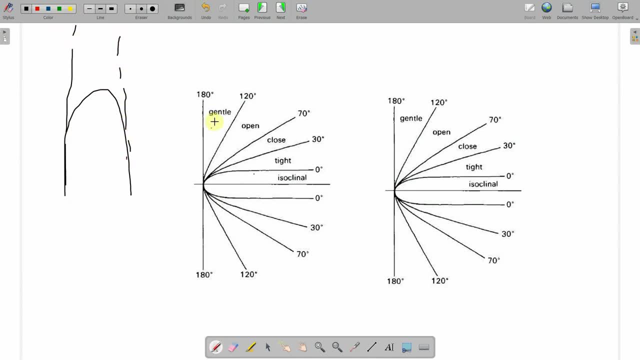 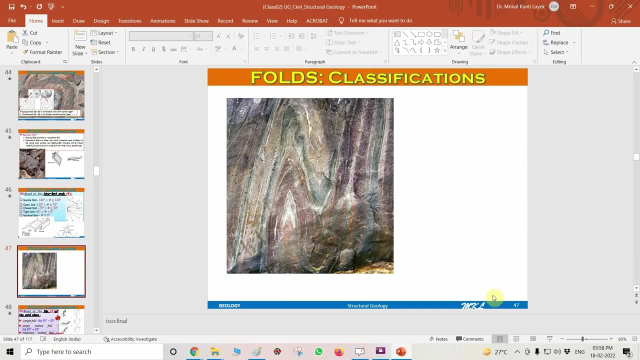 this will not intersect at some point, or it might intersect at low angle, So that type of fold is called isoclinal fold. So what is? what type of fold is this, This one Plus? So what's the angle it's making, The interleave angle? 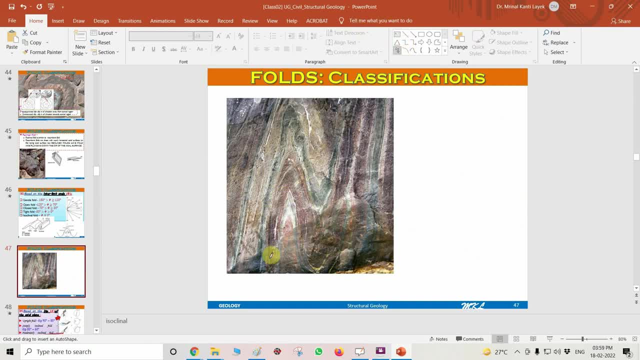 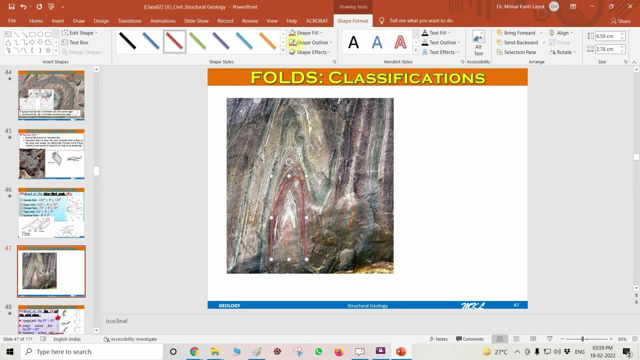 If you draw it. So that's the strata. If you draw the interleave angle, then what will be? If you draw it from here? It is very near to 0 degree, 0 degree, So it's isoclinal fold. 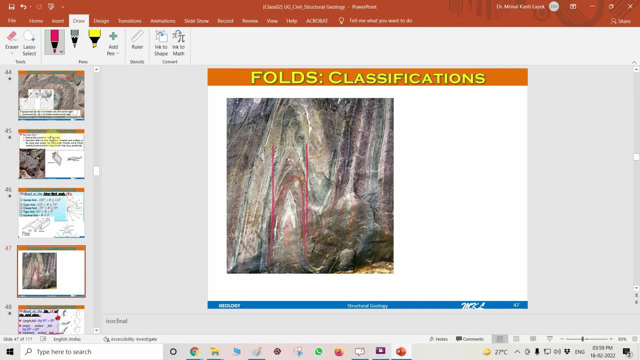 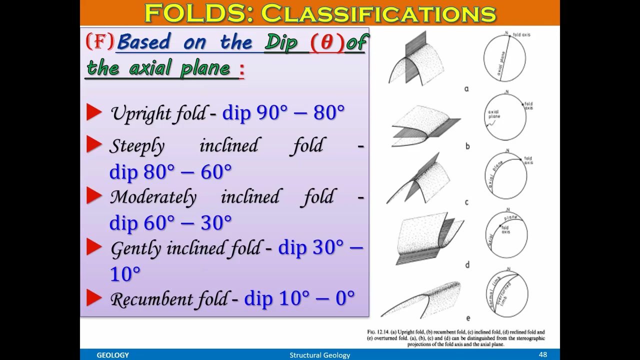 Very near to the 0 degree. See, in nature you will not get the actual 0 degree, But it's kind of giving you the sense That is isoclinal fold Now based on the depth of the axial plane. 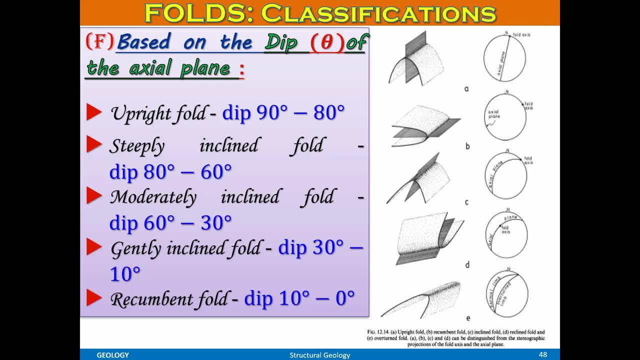 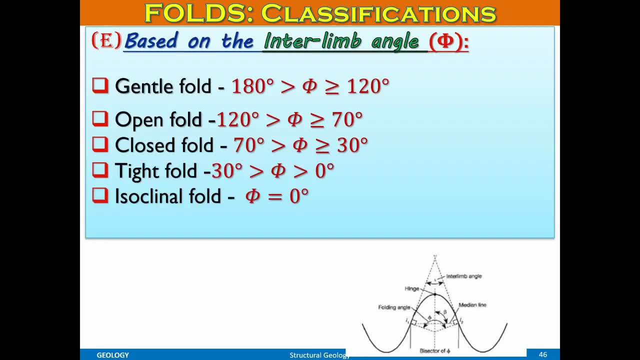 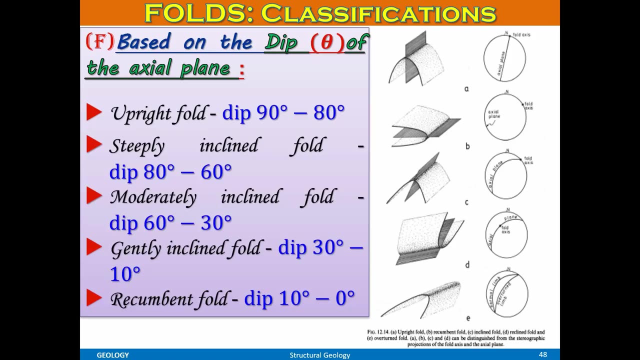 remember. So we have classified fold on the basis of what? On the basis of? On the basis of interleave angle? Now I am classifying the fold on the basis of depth of the axial plane, Or the axial plane orientation. 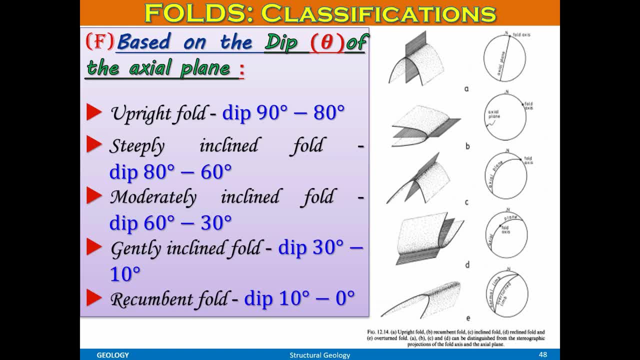 How is your axial plane oriented? Depending on that, you are classifying the folds. So first one is the upright fold. So this is your upright fold, Where you can see the axial plane is vertical. Okay, When the axial plane is vertical, 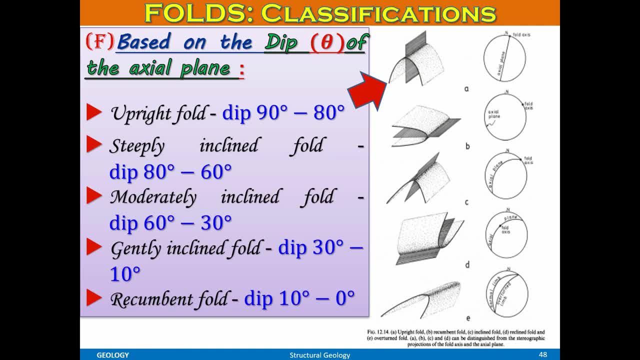 the axial plane is almost vertical. I mean the depth could be within 80 to 90 degree. Then you will be saying it's a upright fold. These are very general terms used in geology. Okay, So you should know about this. 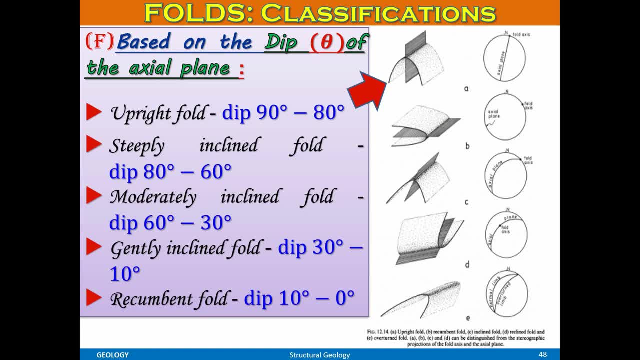 That the upright fold. Upright means it's a perpendicular. The axial plane is almost perpendicular to the horizontal plane. Now, steeply inclined fold could be when the depth is almost 80 to 60 degree. Then I can classify another classification. 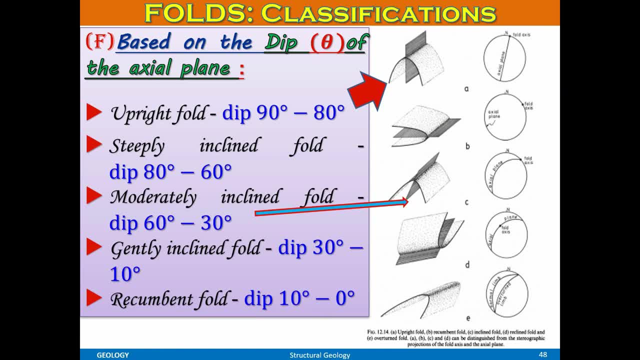 That moderately inclined fold. That depth is 30 to 60 degree. And there is another fold That's called the gently inclined fold. By seeing this photograph, I think you got the idea. Now you incline this axial plane to 10 degree. 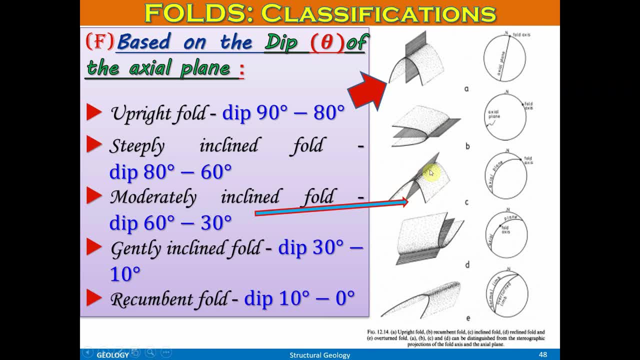 Then you will get the gently inclined fold. Okay, Fifth one is the recumbent fold. When the depth is from negligible amount to 10 degree, then you will have the recumbent fold. So where is the recumbent fold here? 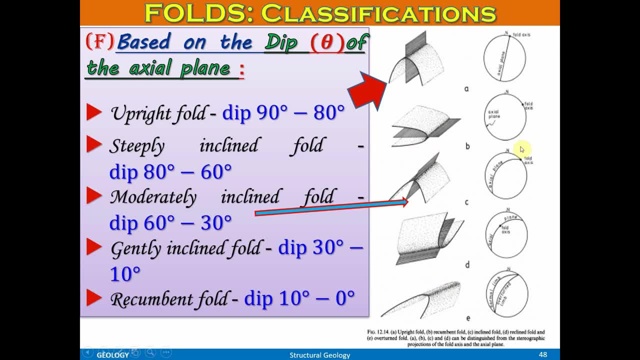 Where is the recumbent fold among these five? Where is the recumbent fold When the axial plane is at 0 degree? If this is 90 degree, which one is the 0 degree? So A, B, C, D, E, tell me. 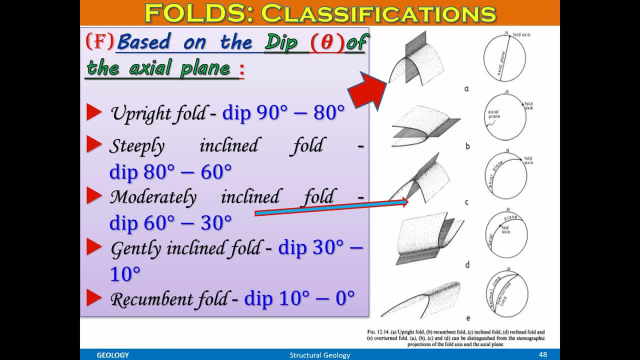 Which figure is giving you the sense of recumbent fold, Or which is the schematic diagram of the recumbent fold? Which one Tell me? This one is very simple, Okay, So the axial plane is drawn. So in recumbent fold, the depth is from 0 to 10.. 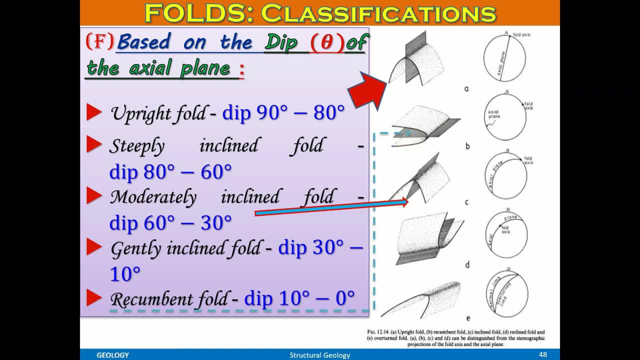 Means it is nearly horizontal. So this one could be your recumbent fold, This one. Now another two-fold diagram. you can see here that first one is the recumbent fold. So what is a recumbent fold? 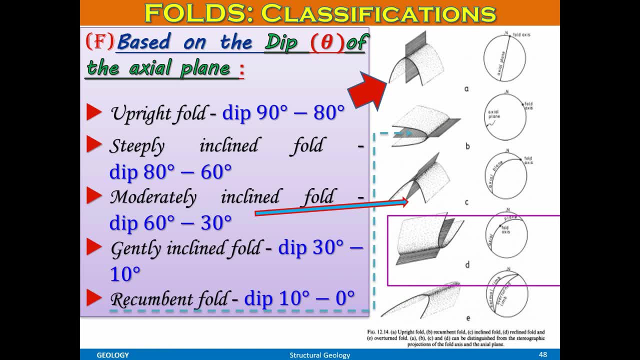 I just discussed in the last slide. So what do you mean by recumbent fold? See, these classifications are not given by me. It is given by Clifty, 1964.. So he has basically classified this. So what do you mean by recumbent fold? 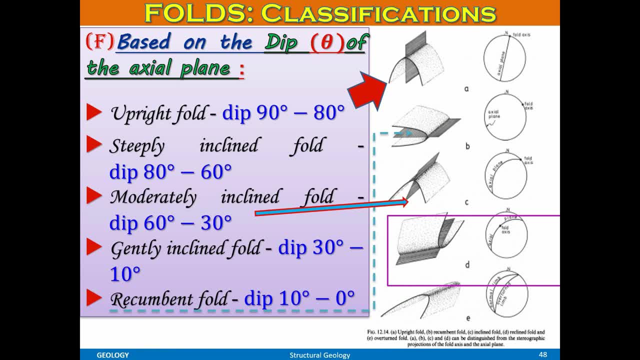 Class And another type of fold you are seeing here at the below bottom. Which type of fold is that? So this is the overturned fold. i'm not going to explain what is the overturned fold. go through the materials otherwise. or go through that book, that bunker book, okay, then only you can understand the problem with you. 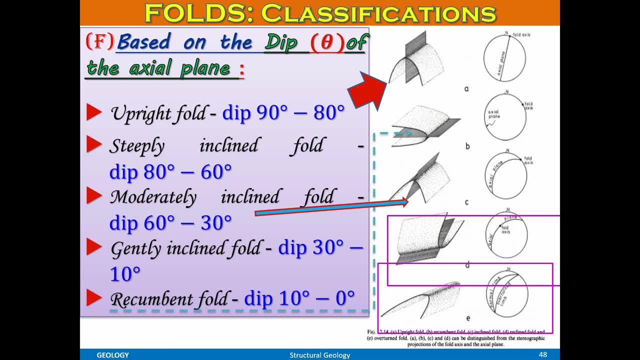 people are that you are not reading. these things are already discussed. so what is overturned for fold? what is reclined fold? i have already discussed. i'm not going to explain it again now. based on the amount of plans of the fold axis, you can also classify uh, depending on the 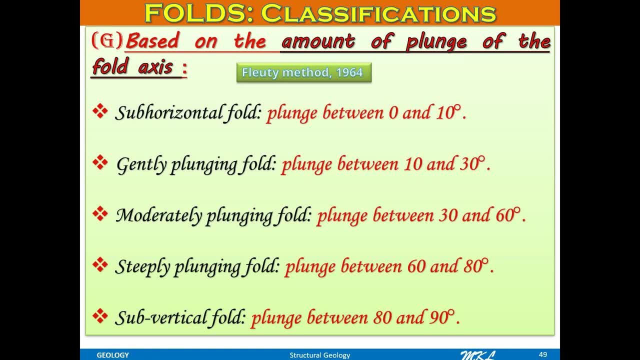 fluidity method. you can classify- and fluidity method is very much uh applicable to understand which type of fold is that? suppose you have a full structure, a full photograph, or you did some structural mapping from there. you can understand, uh, which type of fold it could be from the fluidity. 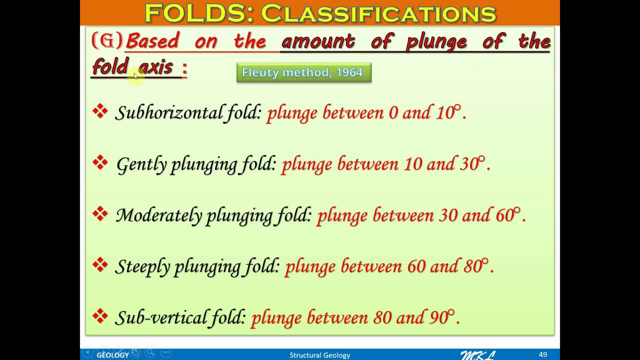 method. okay, so, depending on the plans of the fold axis, yeah, it can be, uh, classified as sub horizontal fold- gently plunging fold- mortality plunging fold- strictly plunging fold. i talked, i'm talking about the flange of the fold axis. now, if i talk about, these two are almost same. that's why i didn't explain it in details. 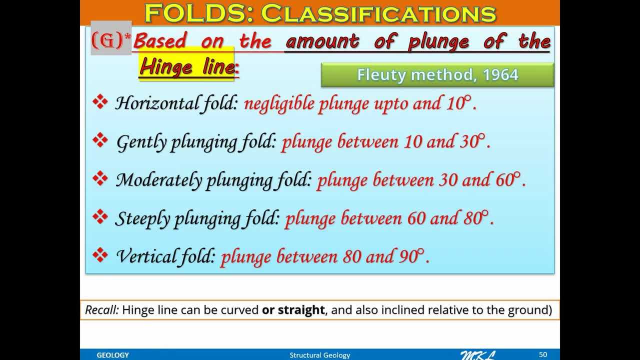 now, if i talk about the amount of plans of the hinge line, now some of you might ask that hinge line could be curved. so how could you estimate the plunging? oh, it could be carved, it could be, uh, have different plunging direction, it could be of different nature. 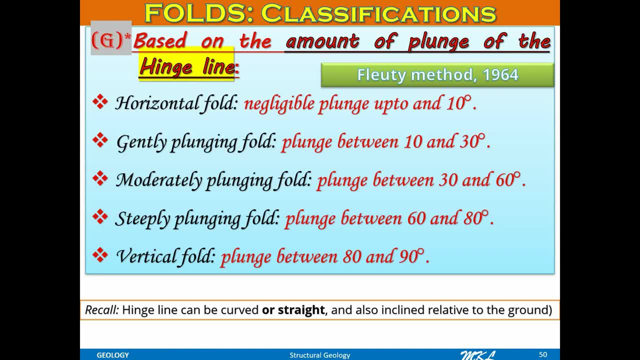 so let's say i'm considering the uh straight line here, so handsome can be curved or straight or it. most of the cases you will find that it influence related to the ground. if the horizontal fold is negligible and plunge is up to 10 degree, then for the horizontal fold your optimal is equal to half degree and if it settle in как. 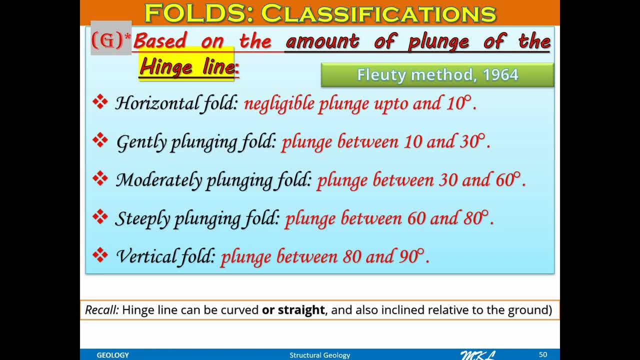 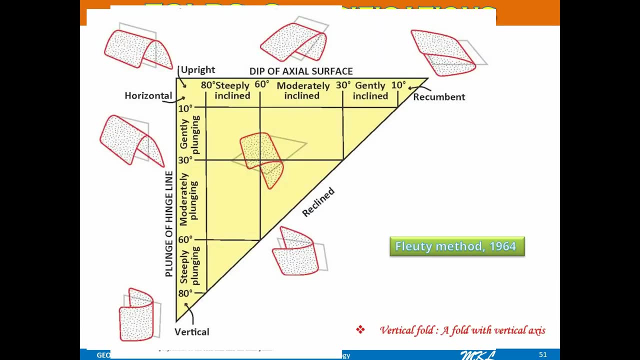 horizontal fold, the plunging is up to 10 degree. for the vertical fold, the plan is in between 80 to 90 degree. in between you have the plunging fold depending on the hinge line. i hope you remembered what is the hinge line now, deep of the axial surface. this is also. this is a diagram for 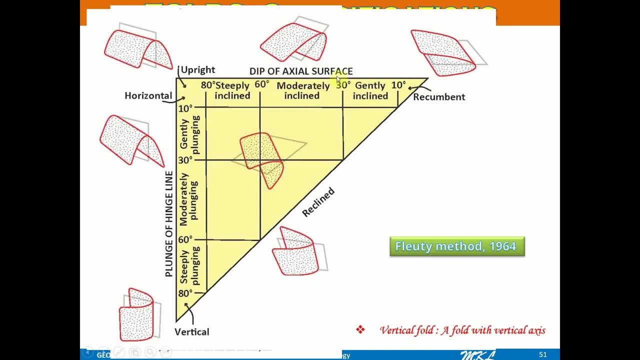 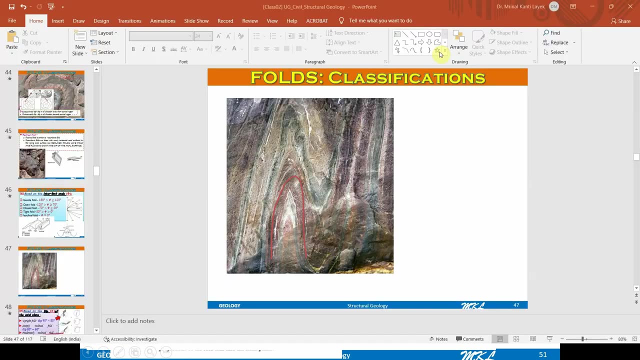 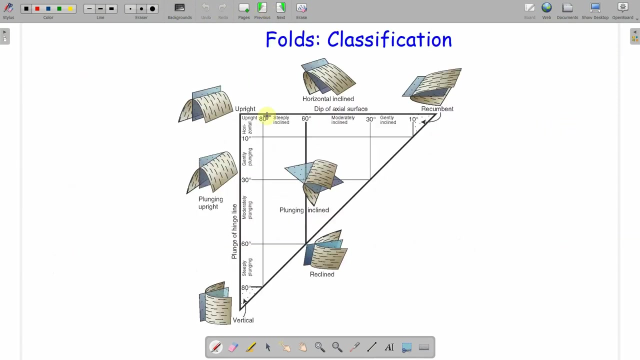 the fluid method, from the, and if you plot deep of the axial surface in this axis and and this vertical axis, if you plot the plunge of the hinge line, then if it's a 10 degree, 0 to 10, you will have the recumbent like this: okay, so it's from the fluid method. and if your tip of the axial surface 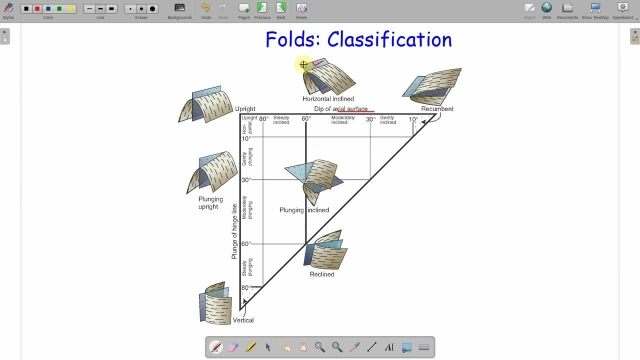 means axial plane. this green or green shade uh plane is the axial plane. this is the axial plane. okay, so this axial plane, if it's horizontal or almost nearly horizontal, then i'll be saying it's a recumbent one. okay, if the dip of the axial 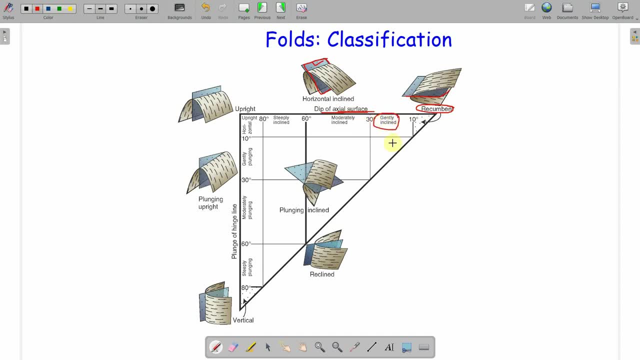 plane is in between 10 to 30 degree. i have already discussed is the gently inclined. now, if the uh axial plane is perpendicular to the horizontal plane or almost perpendicular to the horizontal plane and the angle is 80 to 90 degree, then i will be saying so. it's starting from the zero degree. 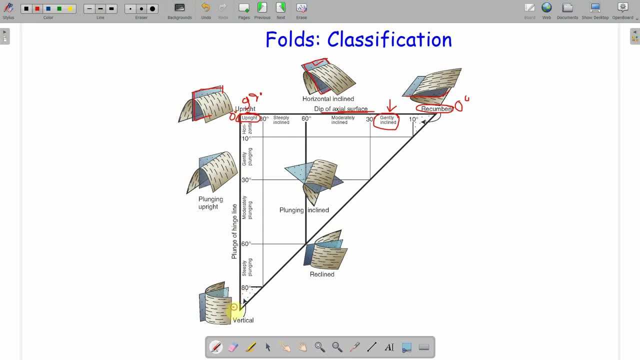 going up to 90 degree, like this, and here the plunge of the hinge line is starting from zero degree and going up to 90 degree. so 0 to 90 degree you are having. so now tell me it's called, what it will be called. it will be called upright. similarly, if the plunge of the hinge line 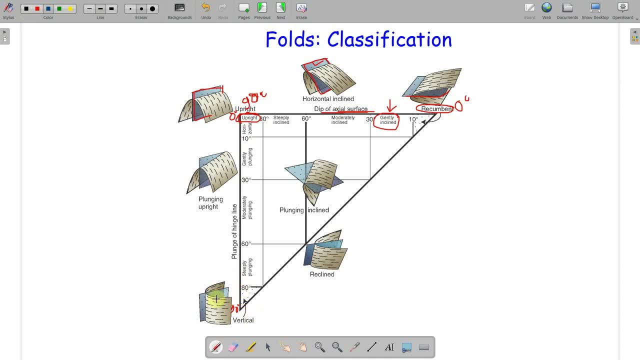 80 to 90 degree, then I will be saying that fold is a vertical fold. So if I draw a folded structure, okay, and this is our axial plane, you are seeing the axial plane is vertical and you are also seeing that the hinge line, that's the hinge line. Hinge line means maximum curvature line on the. 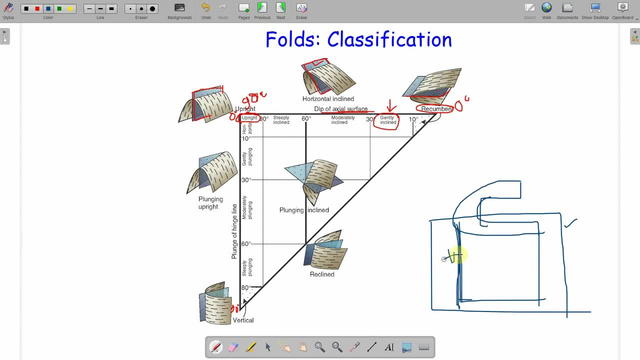 fold surface. okay, So this hinge line H and this is the axial plane S. both are perpendicular to the horizontal. okay, So this type of fold is called the vertical fold or it can be called as, depending on the axial surface orientation, what you can call it. 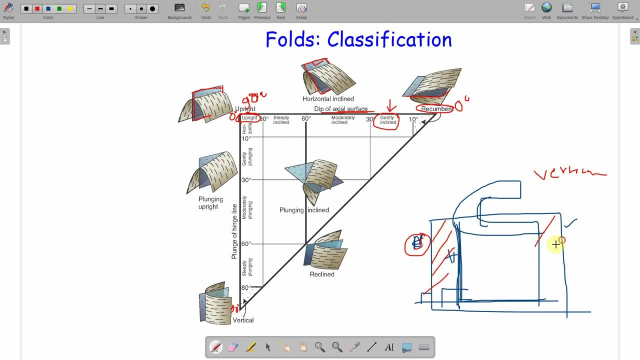 As the axial surface is, or axial plane is vertical, what you can call it this fold, what you will be calling this fold. So it's a vertical fold, and it will be also which one? yes, it's also upright fold. So your section B. one student from section B, he. 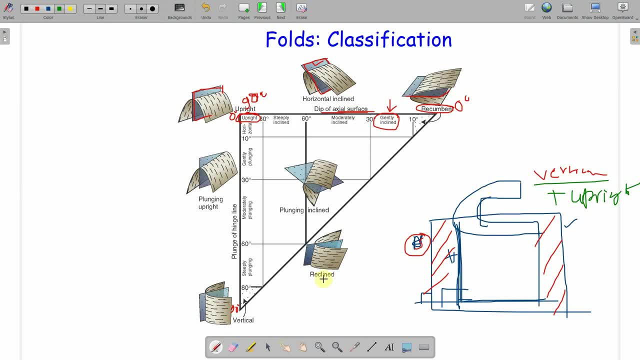 was asking that: is it possible to have the upright and vertical fold together? and it's quite possible. From this diagram you can see that 90-90.. That's the structure. okay, now there is another fold drawn here that's called a reclined fold. So what do you mean by recline fold? I have discussed where the axial surface or 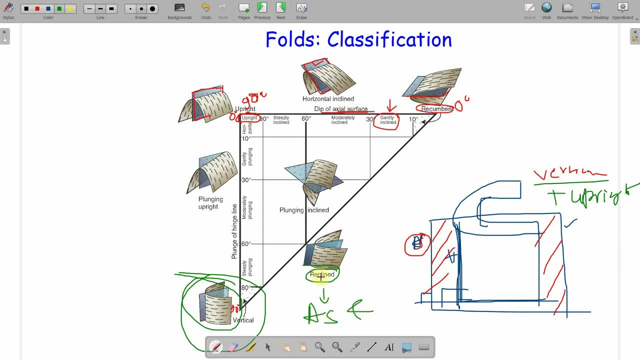 the axial plane and the hinge line- forfor now let's consider it's a hinge line, straight hinge line- are in the same messages as in the external holding. the vertical fold h changes the arc until its smallest and the shaft of happen direction. so these are dipping in the same direction. so in which point you? 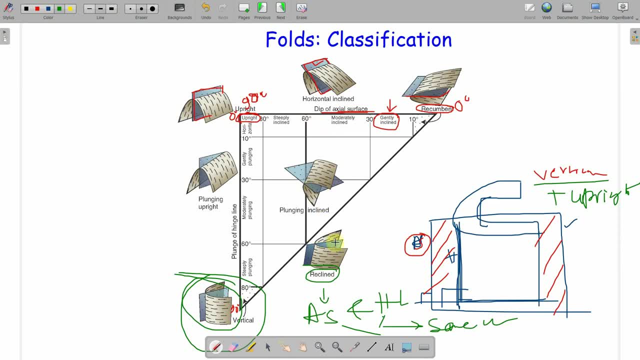 will have that, the that thing, at which point you will obtain at this point and again at this point. so here you can see, the plunging is 60 degree and dipping is also 60 degree. so then it's a reclined here also, you will be seeing that. 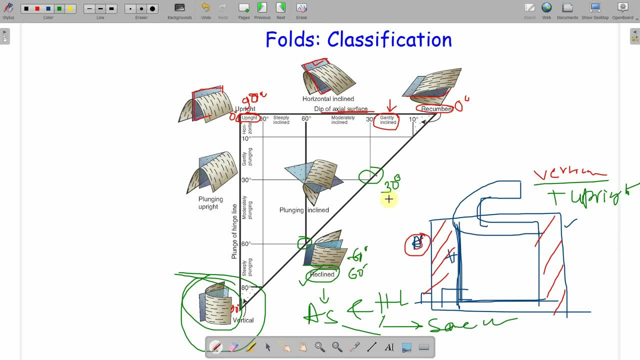 plunging of the hinge line is 30 degree and dipping of the axial plane is 30 degree. so here also you can get one reclined fold structure. okay, now another example has been presented here that you can see that if the plunge of the hinge line is 30 degree- see plunge of the hinge line is 30 degree and deep is deep of. 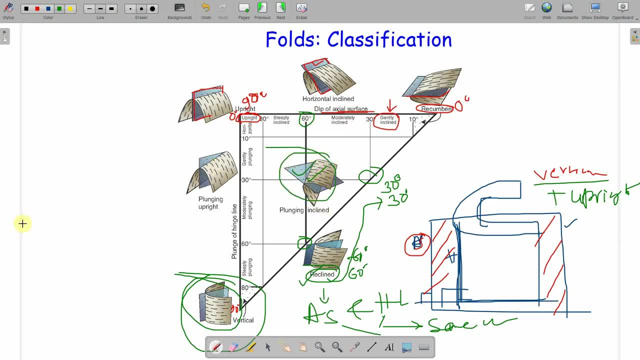 the axial surface is 60 degree, then the fold will look like this: so the fold, or the classical one I used to draw, or I am drawing from the class one that I was drawing, that upright fold, okay, upright horizontal fold. so if I, if I want to specify it on the basis of these two parameter, then I will be saying it's: 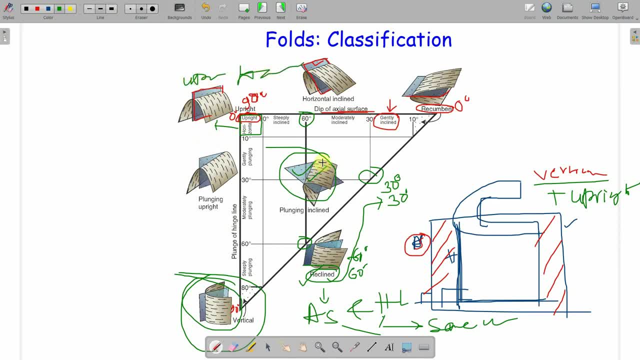 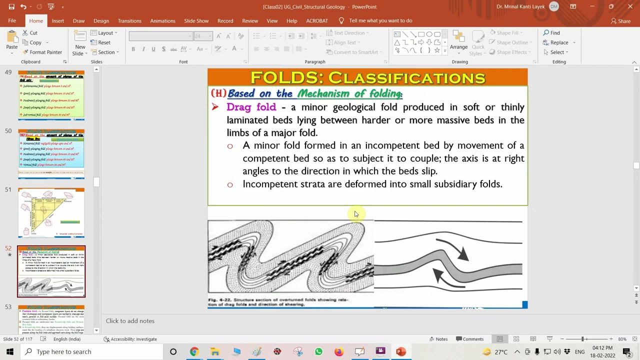 a upright horizontal fold because the hinge line is horizontal. and why upright? because the axial plane is perpendicular to the horizontal plane, that's right upright. now, based on the mechanism of folding, the fold can be classified into mainly three types. first one is the drag fold. so to understand that, 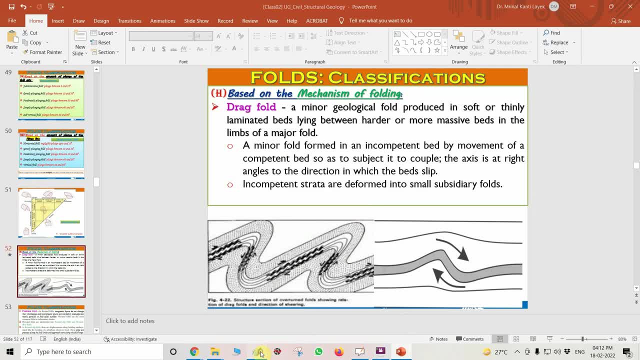 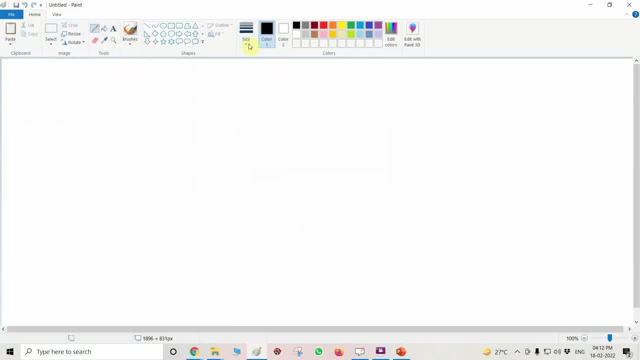 drag, fold. let us, let us consider two things, that let us consider there is a horizontal strata, okay, and in between two, where this layer, this layer number one, this is layer number three and this is our layer number two, two, okay, so this is one, two and three, and I'm 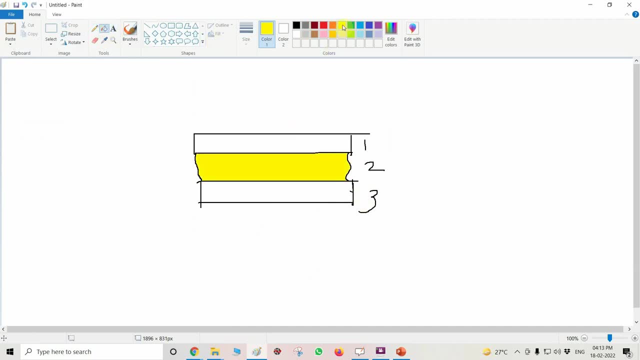 assuming layer three is incompetent comparing to layer one and layer two. okay, so what will happen if you give lateral pressure to create a fold? then what will happen? the folded part due to the presence of the lateral pressure, the competent layer. competent means this layer are the hard rock layer. okay, and 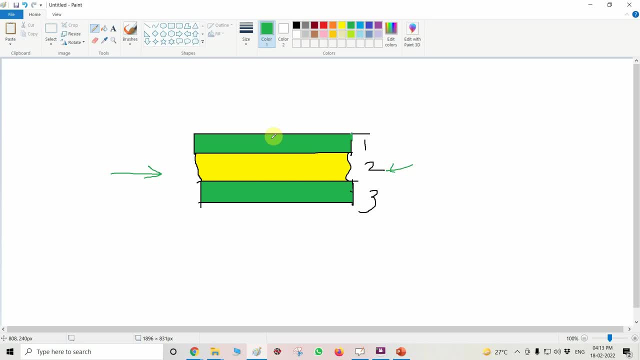 incompetent layers means these are the soft, soft layers. okay, so drag during folding. when a bedding plane slip occurs between the competent and the incompetent layer, then you will find, after giving the lateral pressure, because it can, this yellow zone or yellow layer can be modified into the fold in very different way. 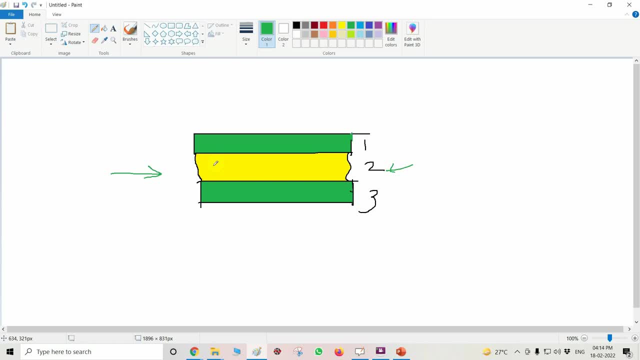 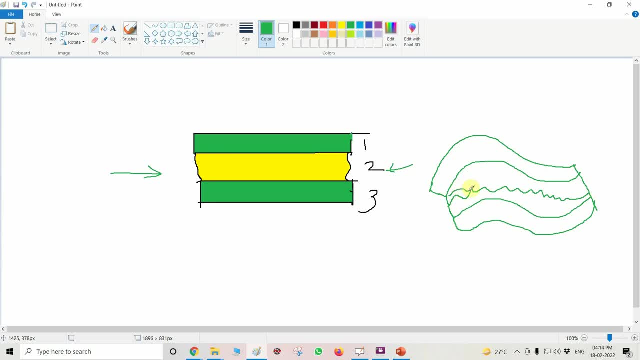 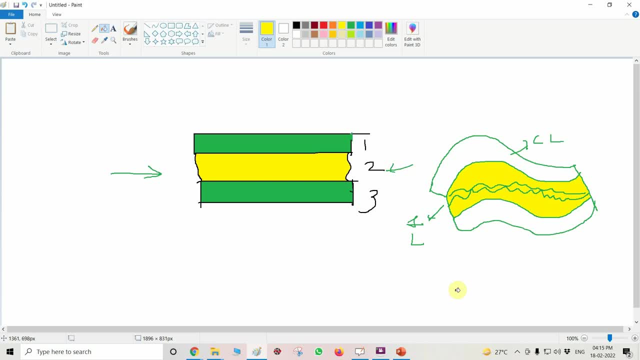 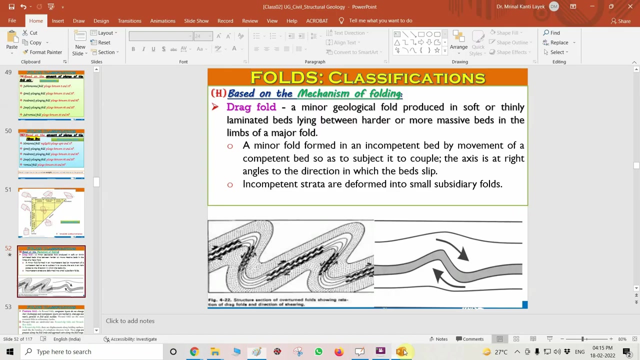 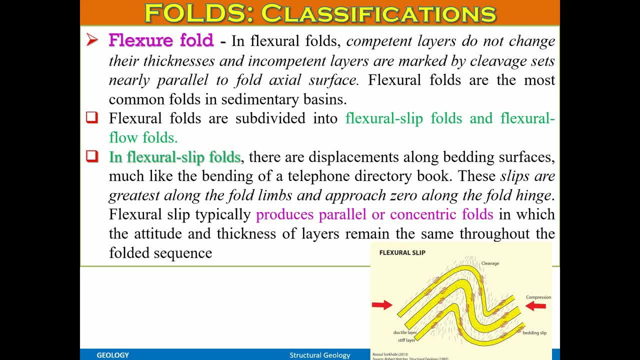 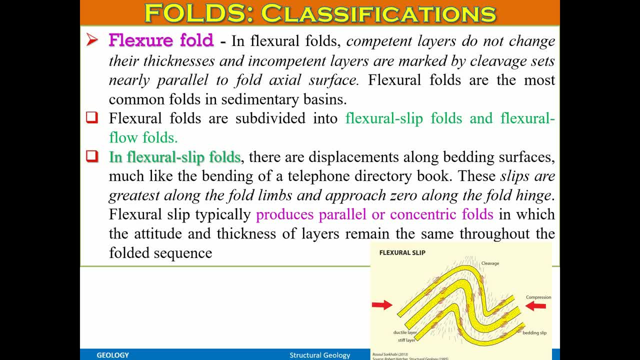 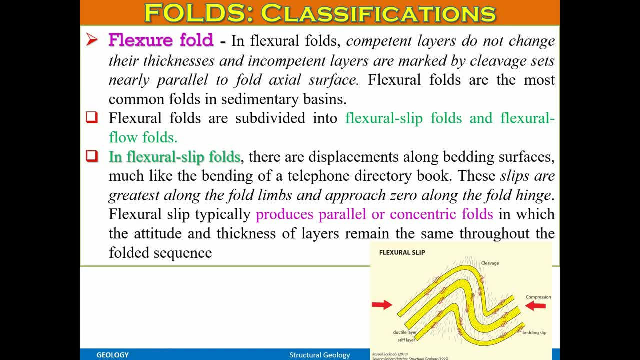 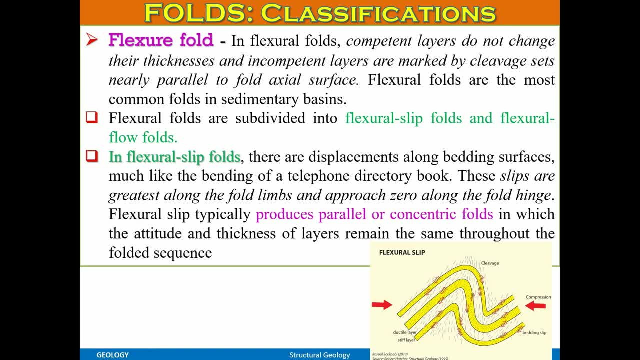 this is what it's gonna end up with26 Nigeria e Ε John, you will be getting- and it will be greatest, it will be larger along the fold limbs and approach zero along the fold hinge. hinge ke side me wo zero ho jayega slip jitna slip hona chahiya ta.